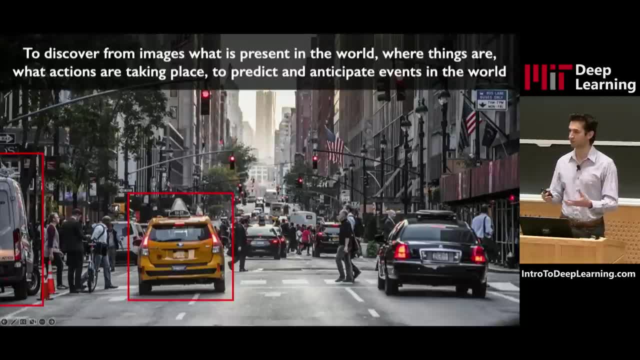 each of these objects at a much deeper level, not just where they are, but actually predicting the future, predicting what may happen in the scene next, For example, that the yellow taxi is more likely to be moving and dynamic into the future because it's in the middle of the lane. 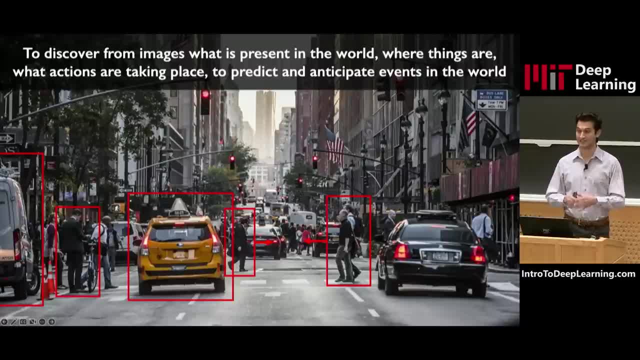 compared to the white van which is parked on the side of the road. Even though you're just looking at a single image, your brain can infer all of these very subtle cues, And it goes all the way to the pedestrians on the road and even these even more subtle cues. 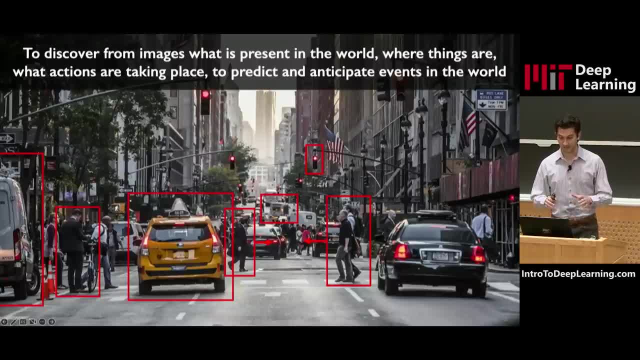 in the traffic lights and the rest of the scene as well. Now, accounting for all of these details in the scene is an extraordinary challenge, But we as humans do this so seamlessly. Within a split second, I probably put that frame up on the slide and all of you within. 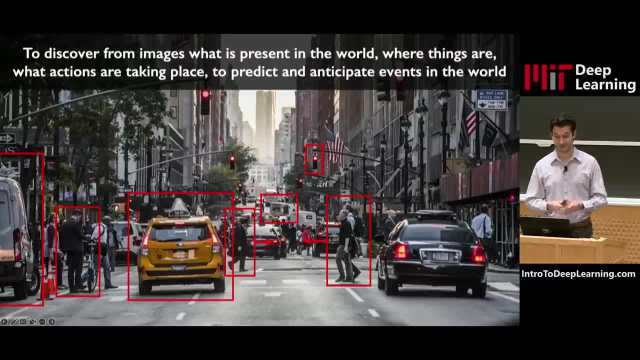 a split second could reason about many of those subtle details without me even pointing them out. The question of today's class is how we can build machine learning and deep learning algorithms that can achieve that same type and subtle understanding of our world And deep learning. 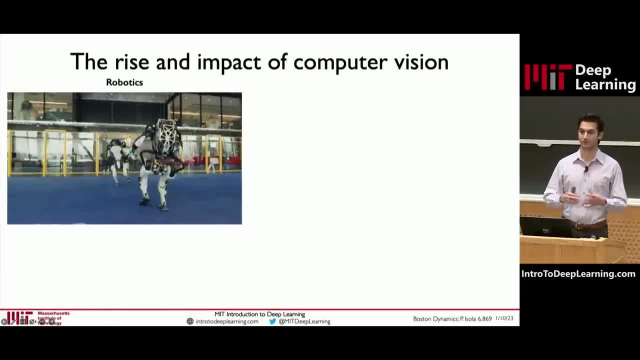 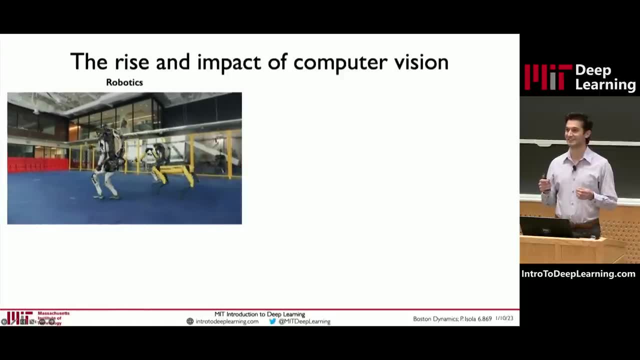 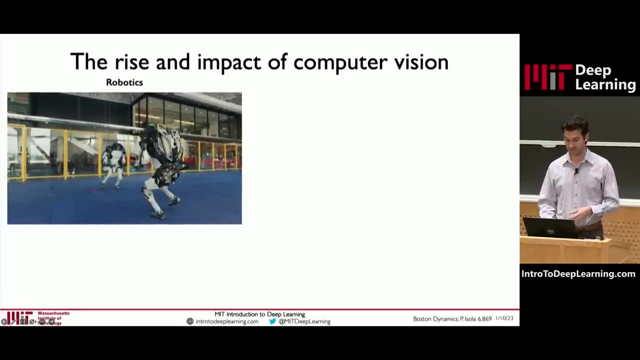 in particular, is really leading this revolution of computer vision and achieving sight of computers, For example, allowing robots to pick up on these key visual cues in their environment, critical for really navigating the world together with us as humans. These algorithms that you're looking at right now are very similar to the algorithms that you're. 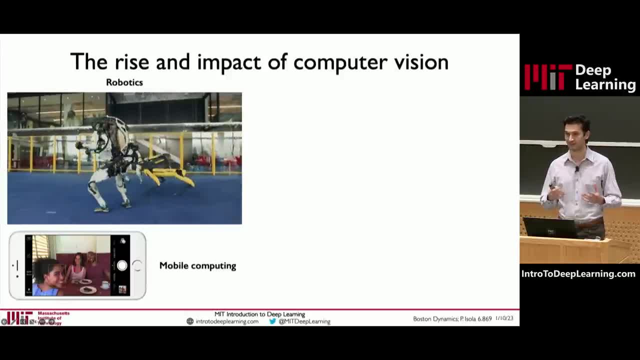 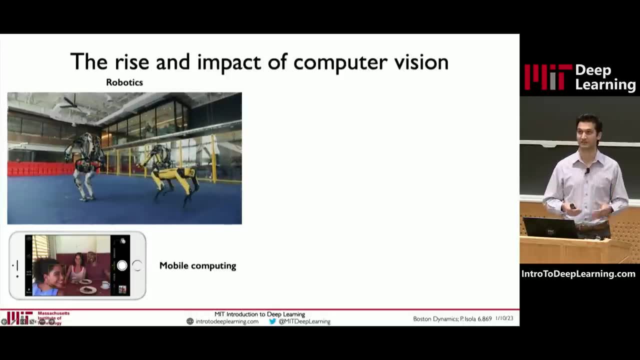 going to learn about today have become so mainstreamed, in fact, that they're fitting on all of your smartphones in your pockets, processing every single image that you take, enhancing those images, detecting faces and so on and so forth, And we're seeing some. 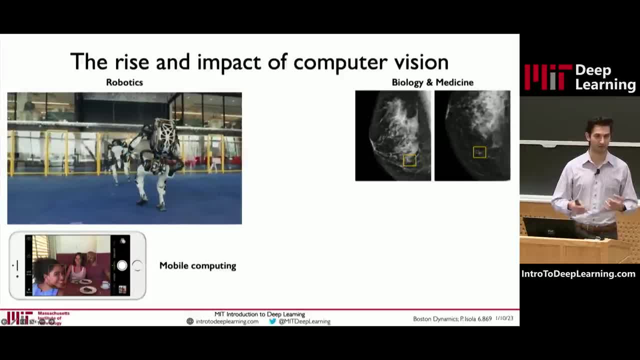 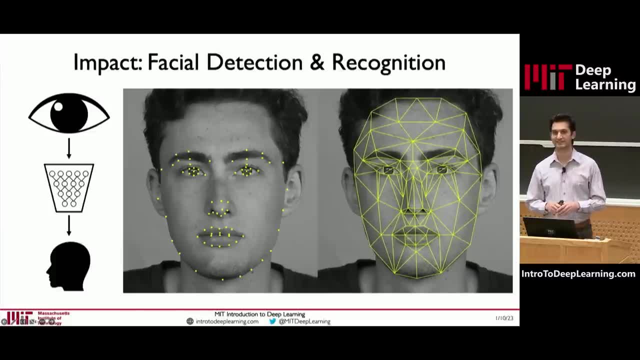 exciting advances, ranging all the way from biology and medicine, which we'll talk about a bit later today, to autonomous driving and accessibility as well. And, like I said, deep learning has taken this field as a whole by storm in the over the past decade or so, because, 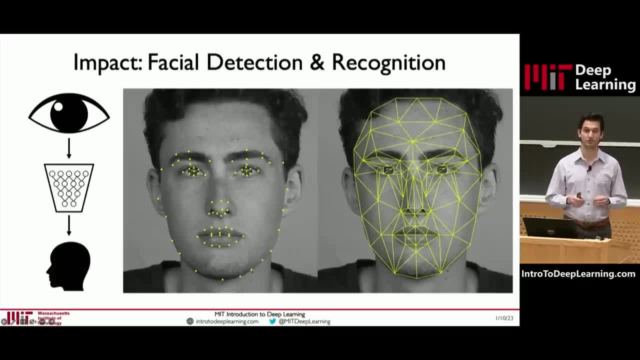 of its ability critically, like we were talking about yesterday, its ability to learn directly from raw data and those raw image inputs in what it sees in its environment And learn explicitly how to perform, like we talked about yesterday, what is called feature extraction. 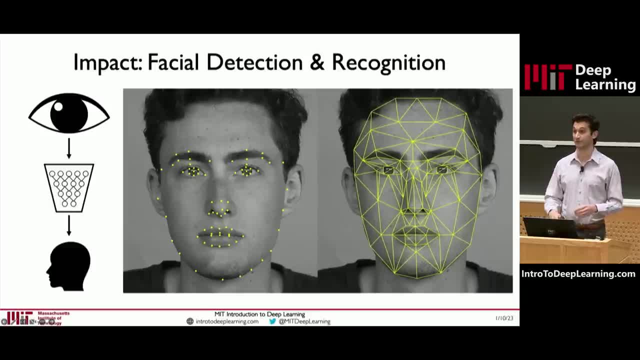 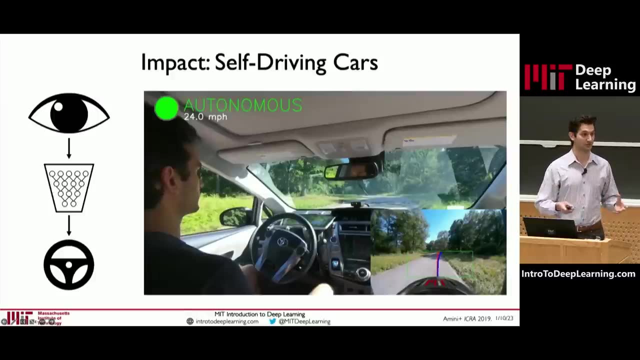 of those images in the environment, And one example of that is through facial detection and recognition, which all of you are going to get practice with in today's and tomorrow's labs as part of the grand final competition of this class. Another really go-to example of computer vision is in autonomous driving and self-driving. 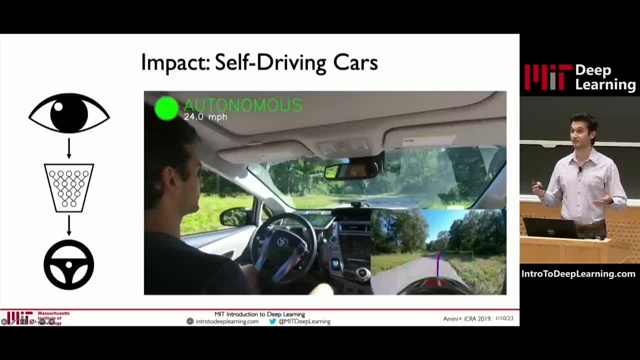 vehicles where we can take an image as input or maybe potentially a video as input, multiple images, and process all of that data so that we can train a car to learn how to steer the wheel or command a throttle or actuate a braking command, This entire control system, the steering. 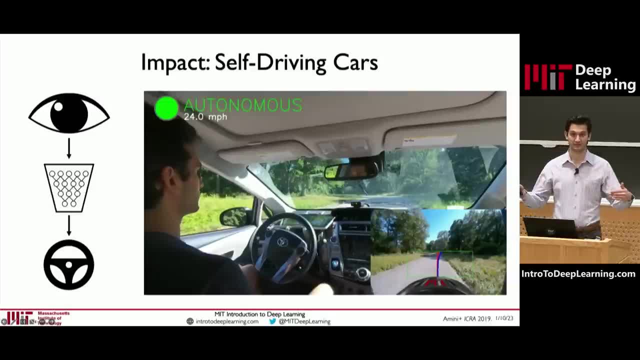 the throttle, the braking of a car can be executed end-to-end by taking as input the images. So we're going to talk a little bit more about that in just a moment, And then we're going to talk a little bit more about how to predict those actuation commands. 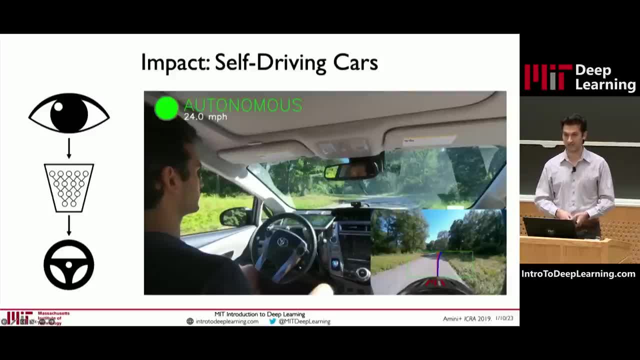 Now, actually, this end-to-end approach, having a single neural network do all of this, is actually radically different than the vast majority of autonomous vehicle companies, Like if you look at Waymo, for example. that's a radically different approach, But we'll. 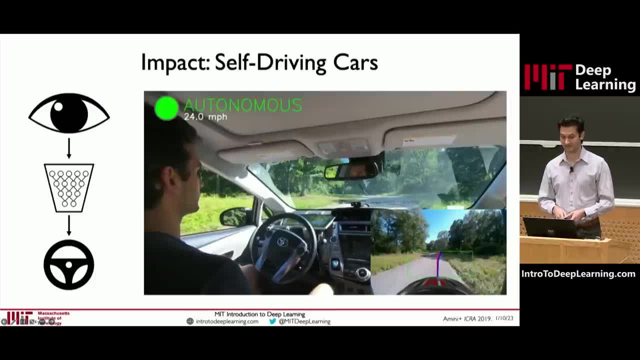 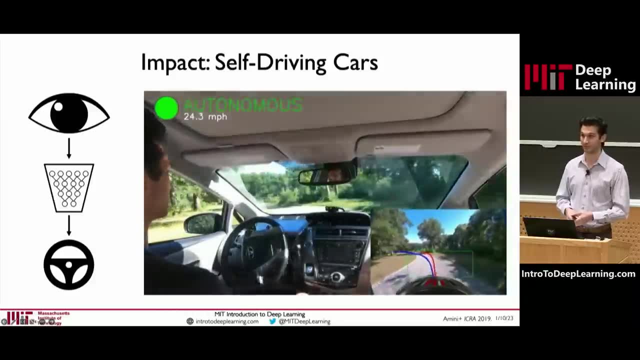 talk about those approaches in today's class, And in fact, this is one of our vehicles that we've been building at MIT in my lab in Cecil, just a few floors above this room, And we'll again share some of the details on this incredible work, But of course, it doesn't stop here. 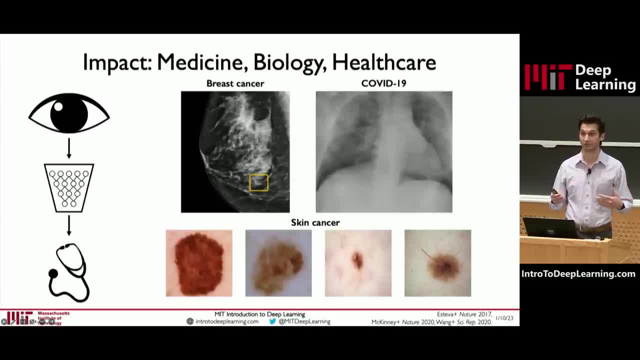 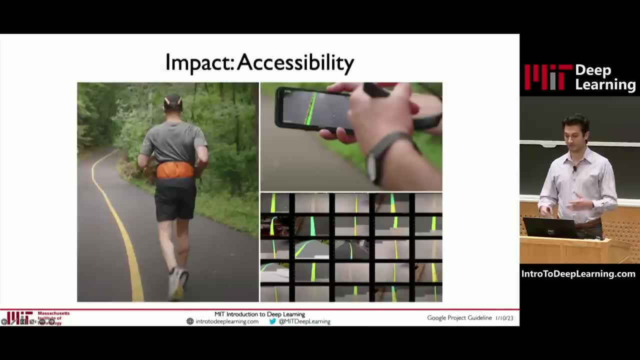 with autonomous driving These algorithms directly. the same algorithms that you'll learn about in today's class can be extended all the way to impact health care, medical decision-making and, finally, even in these accessibility applications where we're seeing computer vision algorithms. 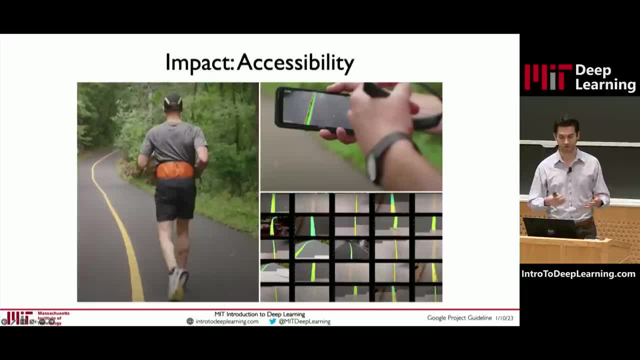 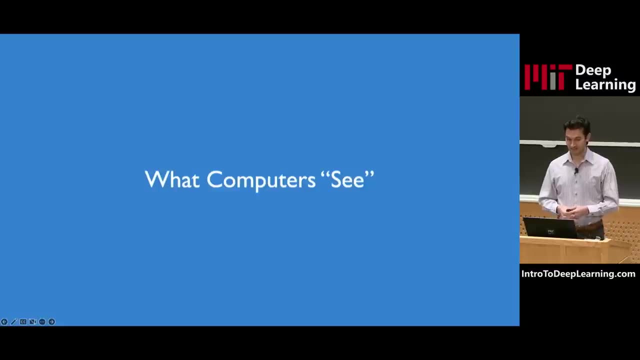 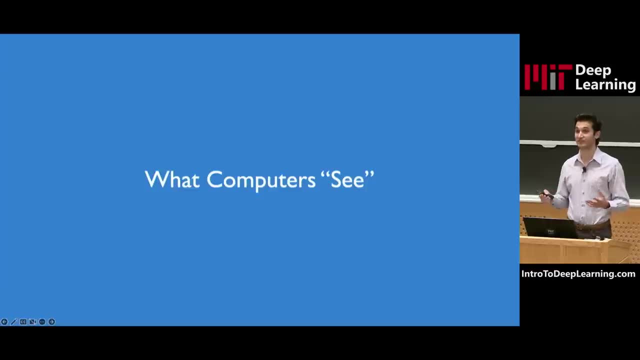 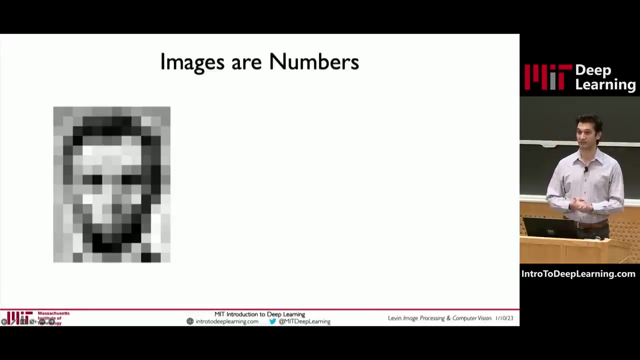 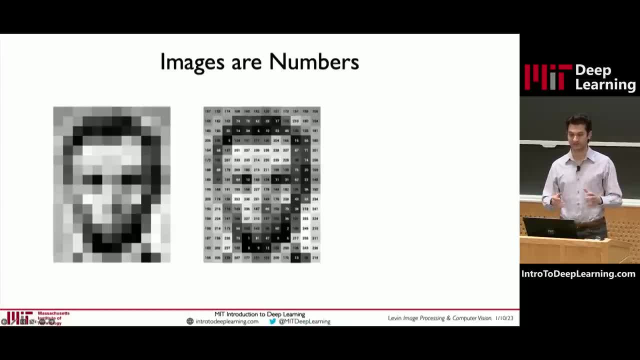 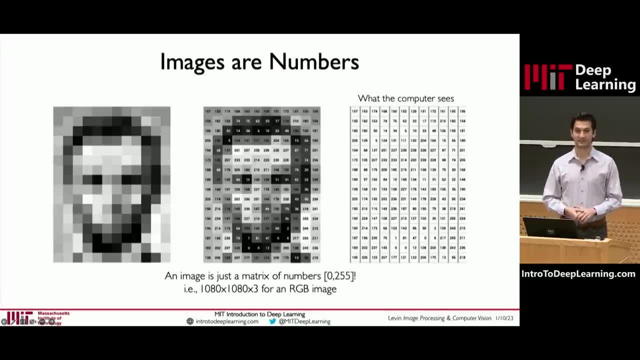 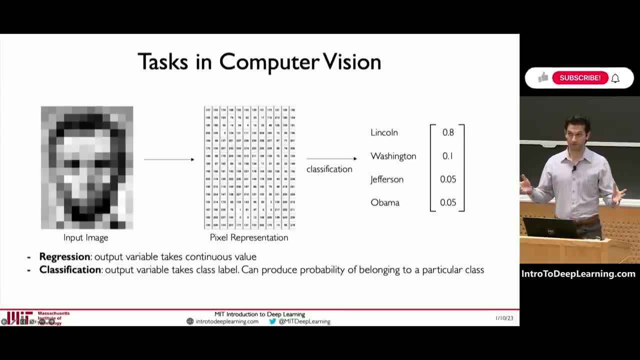 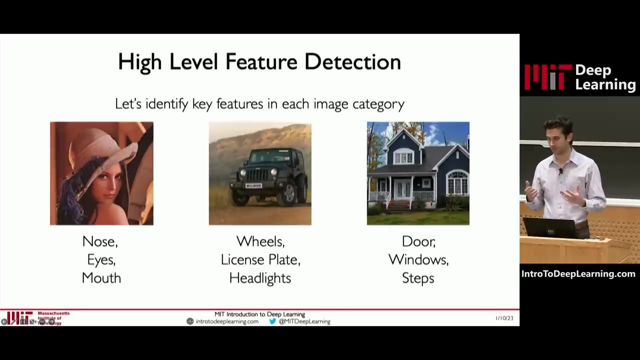 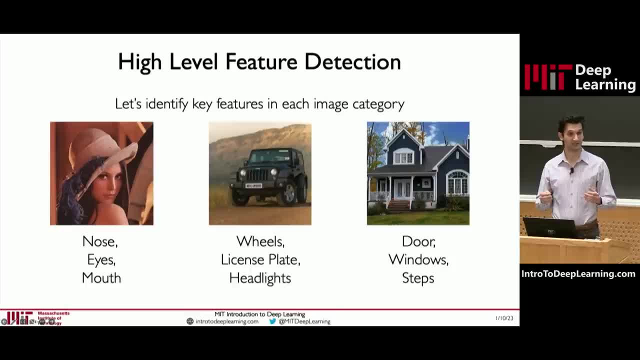 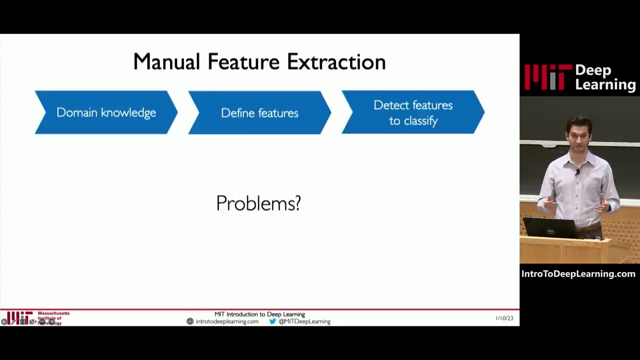 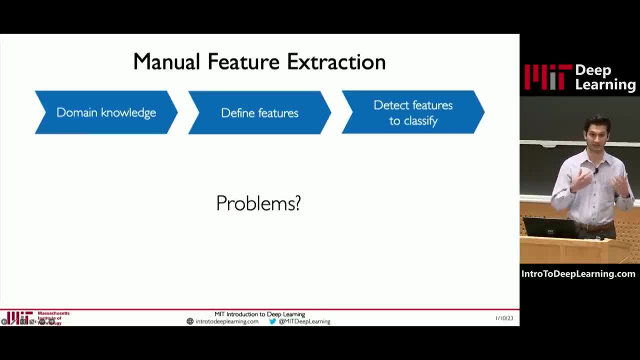 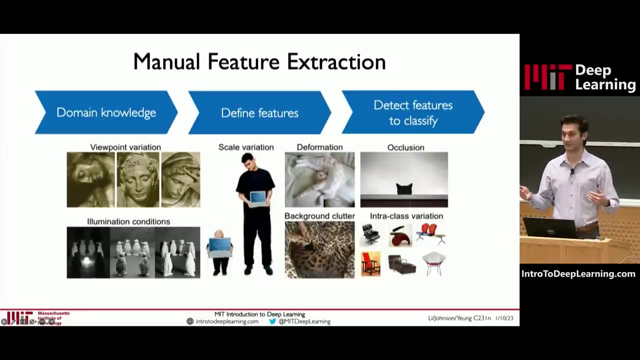 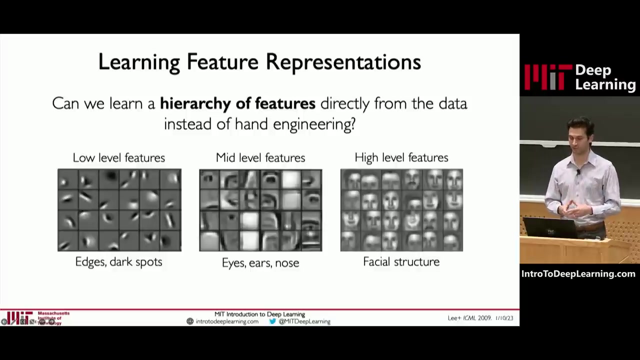 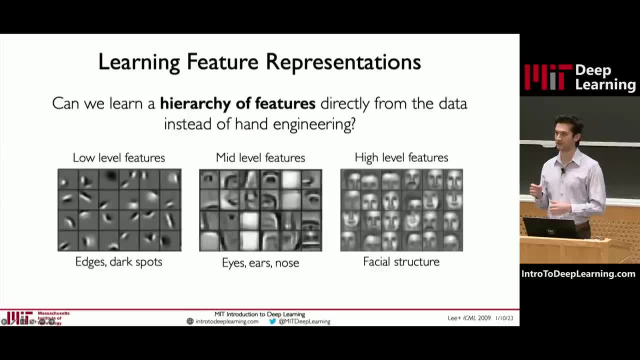 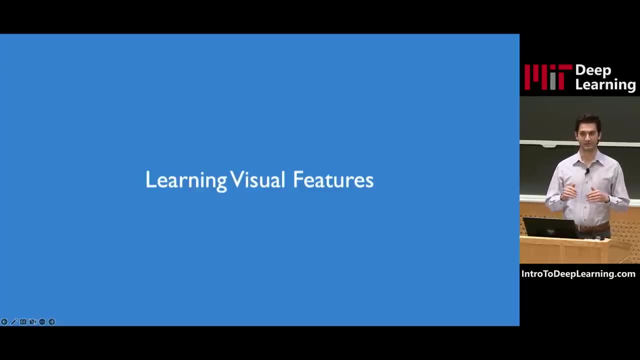 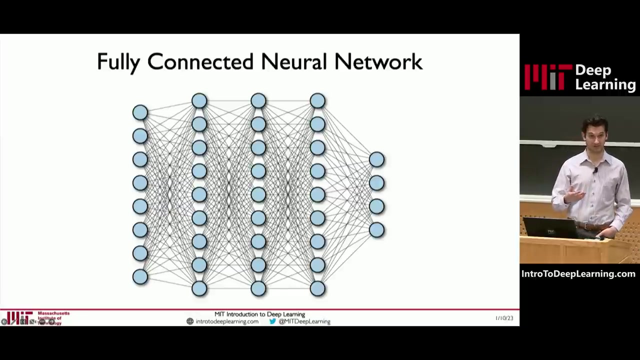 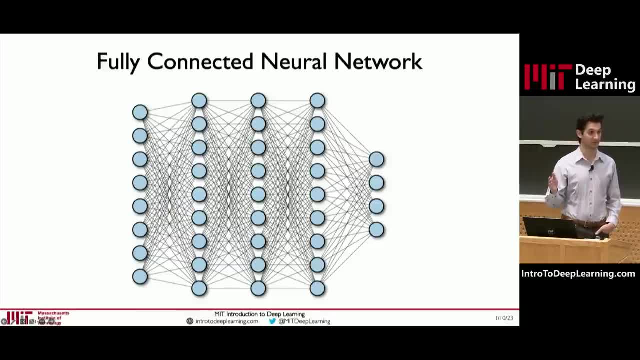 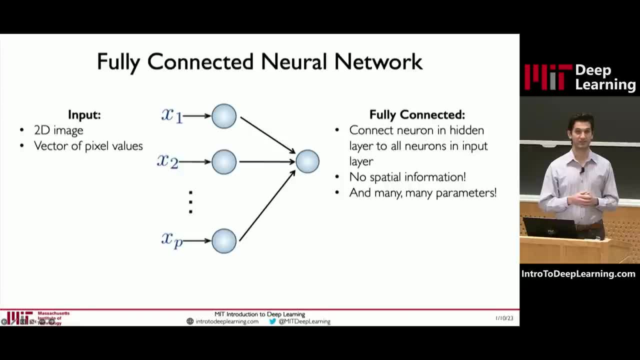 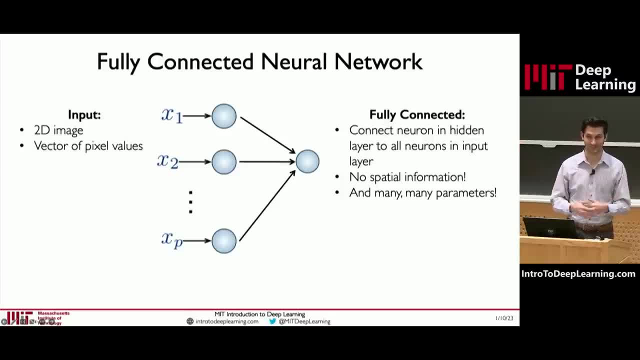 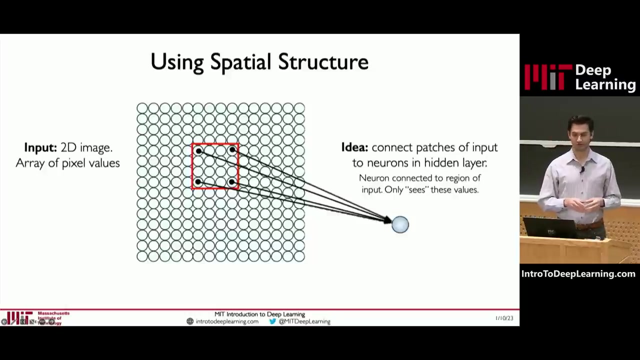 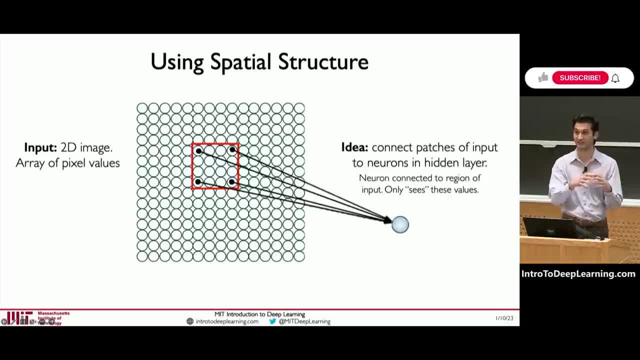 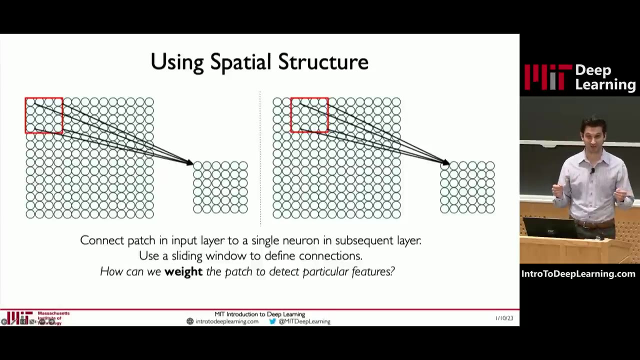 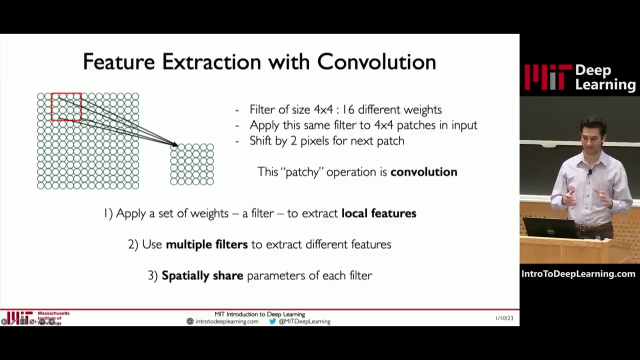 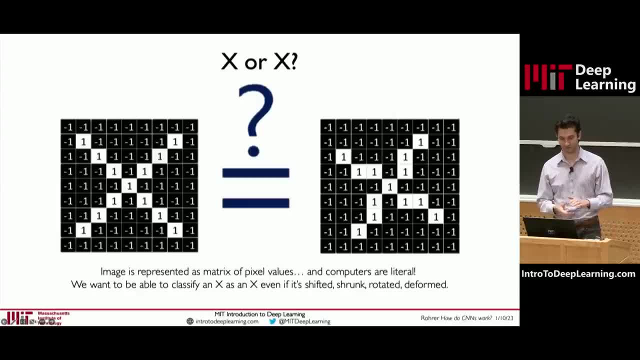 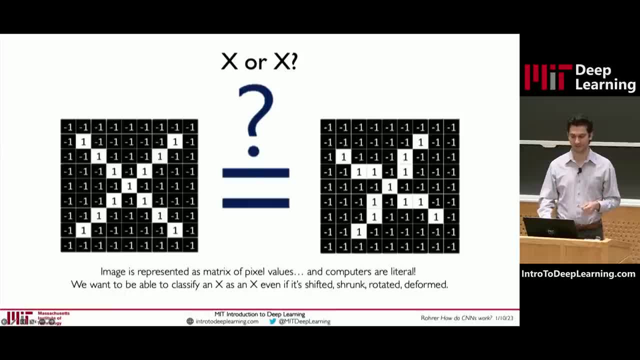 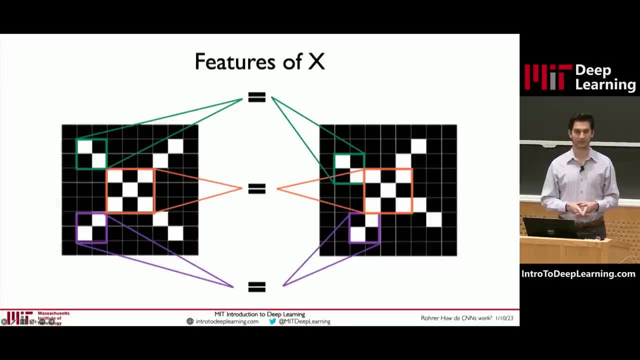 about how we can detect those features that define an X a bit more cleverly. So let's see how we can use convolutions to do that. So in this case, for example, instead we want our model to compare images of this X piece by piece or patch. 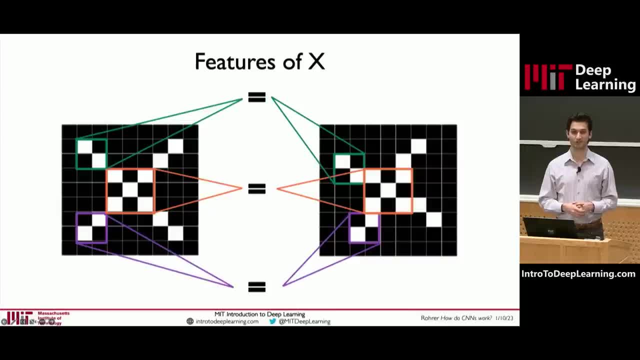 by patch, right, and the important patches that we look for are exactly these features that will define our X. So if our model can find these rough feature patches roughly in the same positions in our input, then we can determine, or we can infer, that these two images are of the same type or the same letter, right? 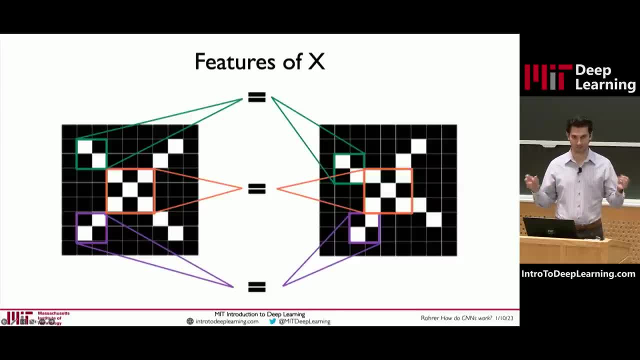 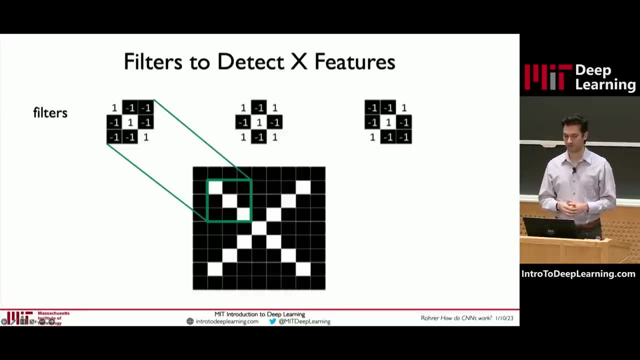 It can get a lot better than simply measuring the similarity between these two images, because we're operating at the patch level. So think of each patch almost like a miniature image, right, a small two-dimensional array of values, and we can use filters to pick up on when these small patches or small images. 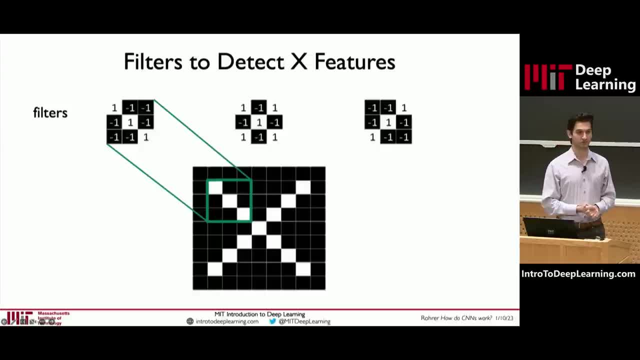 occur. So, in the case of X's, these filters are the ones that we can use to measure the similarity between these two images. So, in the case of X's, these filters are may represent semantic things, for example the diagonal lines or the crossings that capture all of the important characteristics of the X. So, 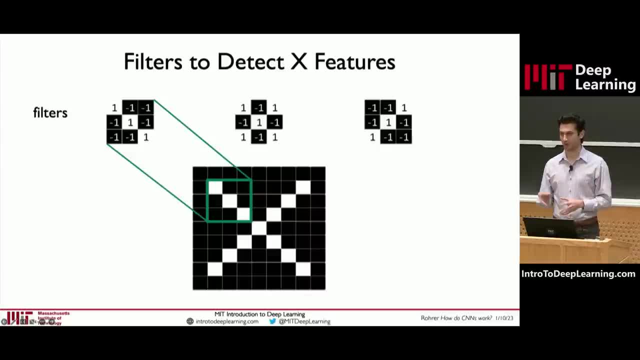 we'll probably capture these features in the arms and the center of our letter, right, in any image of an X, regardless of how that image is, you know, translated or rotated or so on, And note that even in these smaller matrices, right, these are filters of weights, right, these are also just. 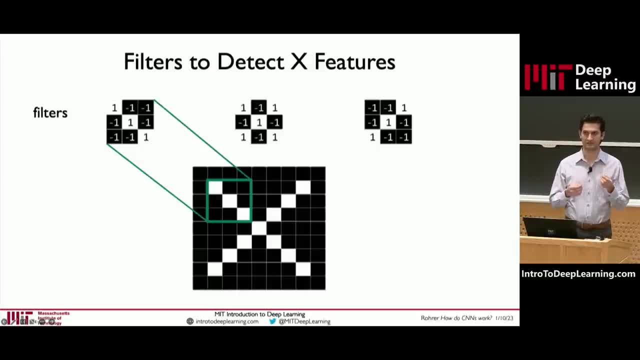 numerical values of each pixel in these many patches is simply just a numerical value. They're also images in some effect, right? And all that's really left in this problem and in this idea that we're discussing is to define that operation that can take these miniature patches and try to pick up, you know, detect when. 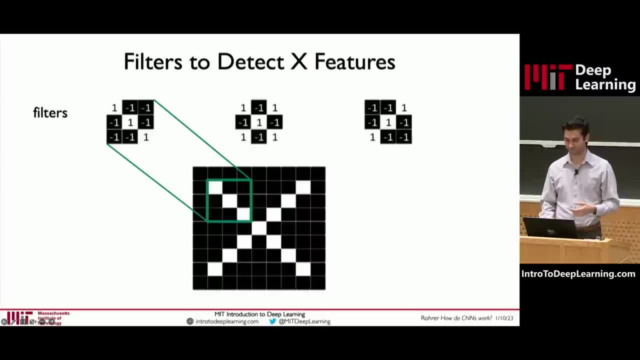 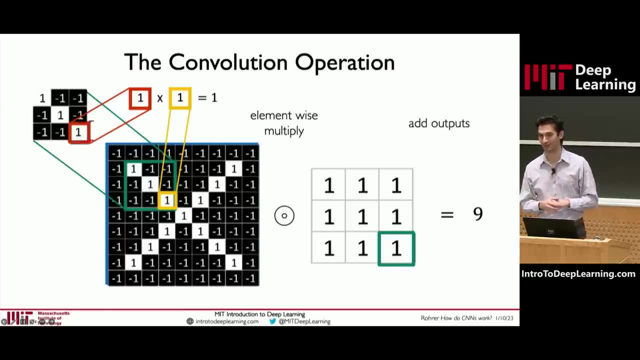 those patches occur in your image and when they maybe don't occur. And that brings us right back to the question of how do we measure the similarity between these two images? So let's go right back to this notion of convolution, right? So convolution is exactly that operation that will solve that problem. 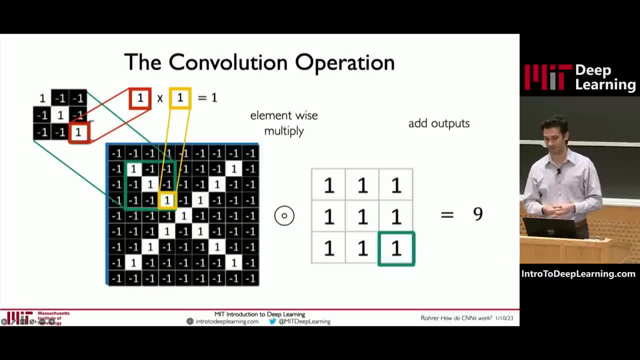 Convolution preserves all of that spatial information in our input by learning image features in those smaller squares of regions that preserve our input data. So, just to give another concrete example, to perform this operation we need to do an element wise multiplication between the filter matrix, those miniature patches, as well as the patch of our input data, And so 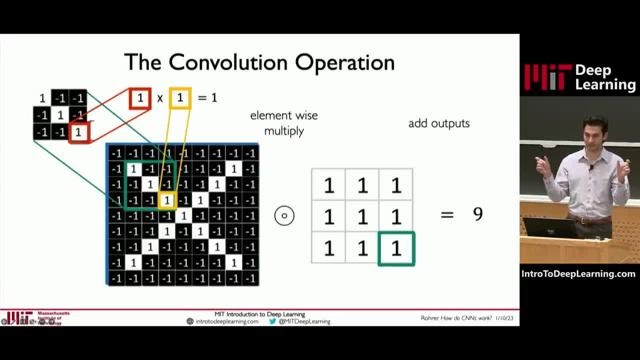 this is basically like a patch of our input image, Right. So you have basically think of 2 patches. You have the weight matrix patch, the thing that you want to detect, which you can see on the top left hand here, And you also have the secondary patch, which is the thing that you are. 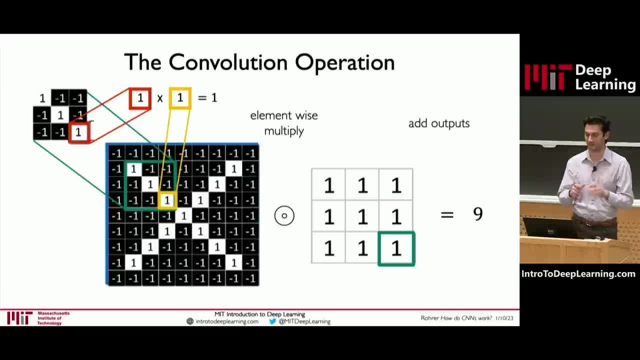 looking to compare it against in your input image And the question is how? how similar are these 2 patches that you observe between them? So, for example, there was this: results in a 3 by 3 matrix as between two small 3x3 matrices. 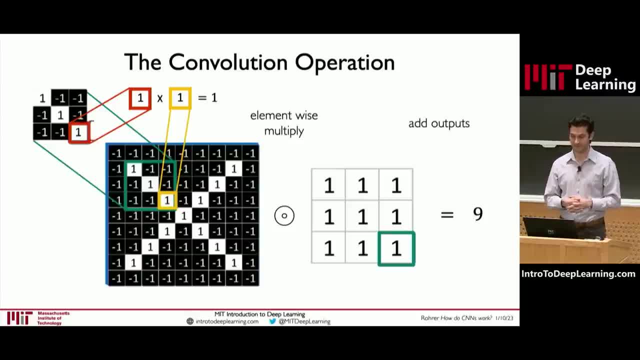 you're going to be left with another 3x3 matrix. In this case, all of the elements of this resulting matrix you can see here are ones right, Because in every location in the filter and every location in the image patch we are perfectly matching. 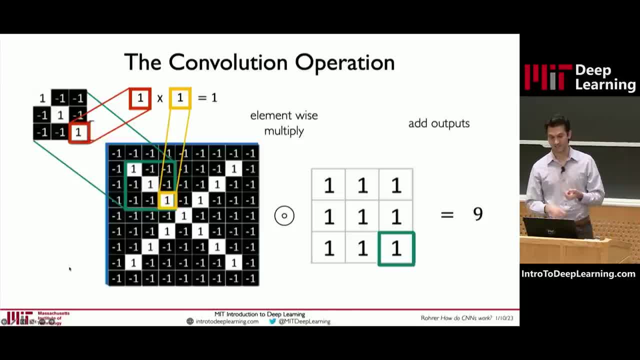 So when we do that element-wise multiplication, we get ones everywhere. The last step is that we need to sum up the results of that matrix or that element-wise multiplication, And the result is, let's say, nine in this case, right? 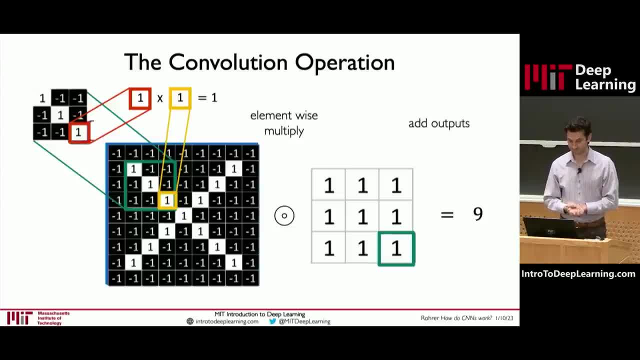 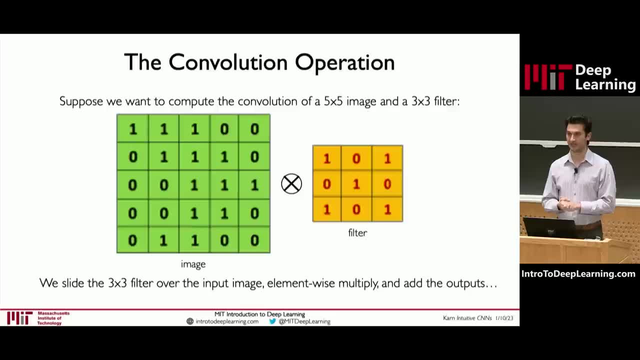 Everything was a one. It's a 3x3 matrix, so the result is nine. Now let's consider one more example. right Now we have this image in green and we want to detect this filter in yellow. Suppose we want to compute the convolution. 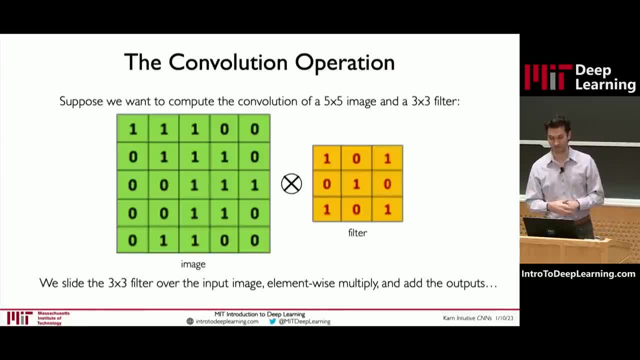 of this 5x5 image with this 3x3 filter. To do this we need to cover basically the entirety of our image by summing up the results of that image. So we're sliding over this filter piece by piece. 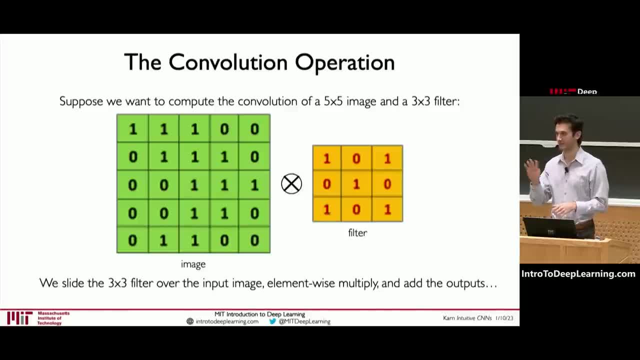 and comparing the similarity or the convolution of this filter across the entire image- And we do that again through the same mechanism At every location we compute an element-wise multiplication of that patch with that location on the image. add up all of the resulting entries. 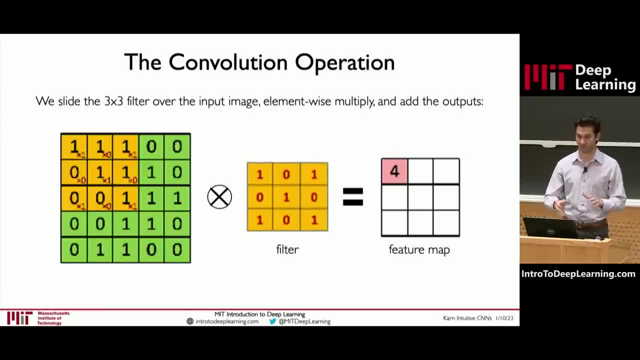 and pass that to our next layer. So let's walk through it First. let's start off in the upper left-hand corner. We place our filter over the upper left-hand corner of our image. We add a new filter, Element-wise multiply. 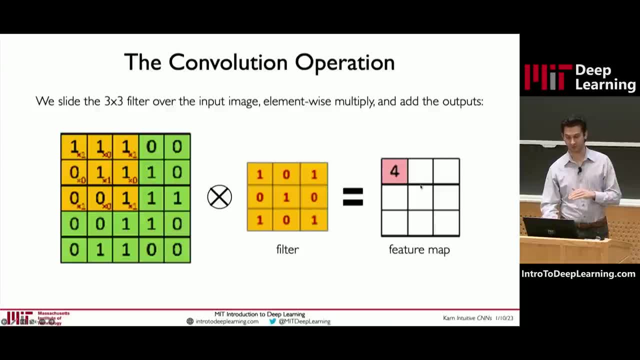 We add up all the results and we get 4.. And that 4 is going to be placed into the next layer. This next layer again, is another image, but it's determined as the result of our convolution operation. We slide over that filter to the next location. 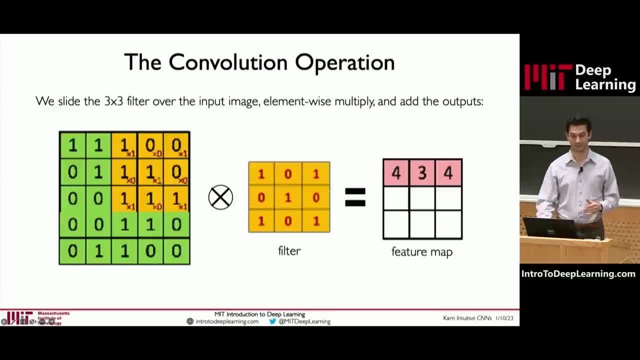 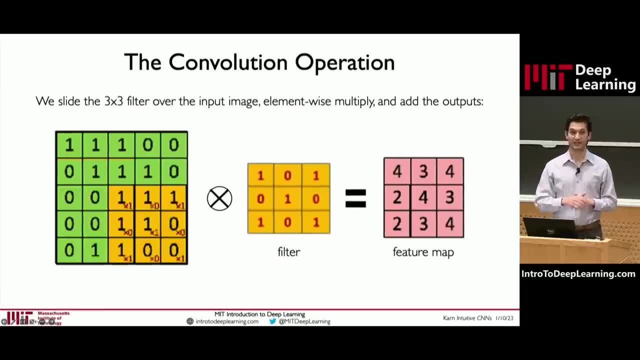 The next location provides the next value in our image, and we keep repeating this process over and over and over again until we've covered our filter over the entire image And, as a result, we've also completely filtered out the result of our output feature map. 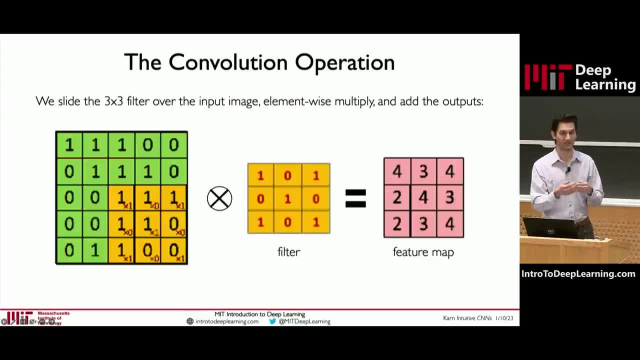 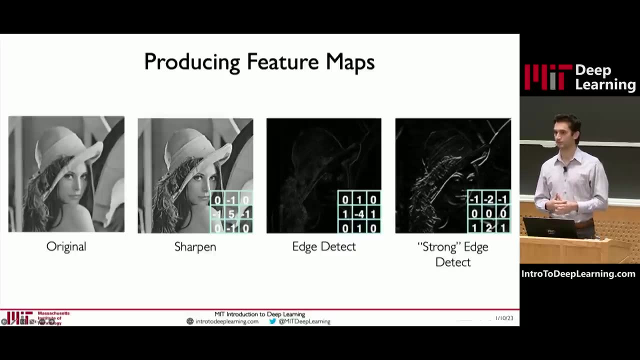 The output feature map is basically what you can think of as how closely aligned our filter is to every location in our input image. So now that we've kind of gone through the mechanism that defines this operation of convolution, let's see how different filters could be used. 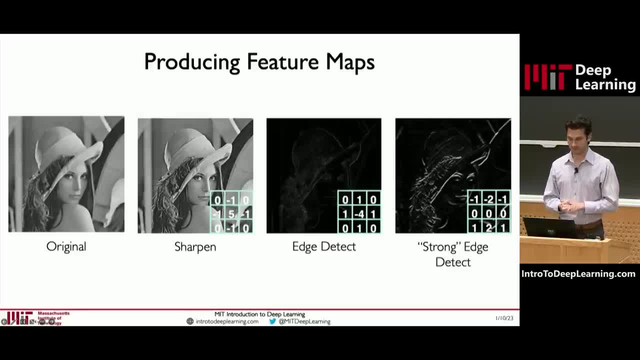 to detect different types of patterns in our data. So, for example, let's take this picture of a woman's face, And the output of a woman's face is a woman's face, And this is a way of applying three different types of filters to this picture. 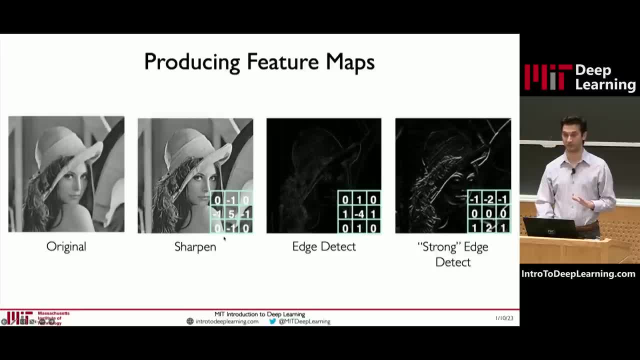 Right, So you can see the exact filter. This is they're all three by three filters, So the exact filters you can see on the bottom right-hand corner of the corresponding face And by applying these three different filters you can see how we can achieve drastically different results. 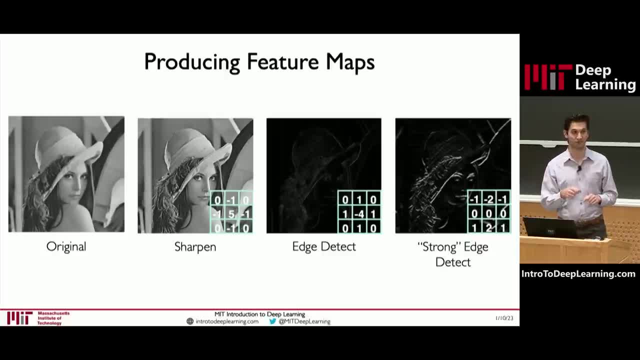 And simply by changing the weights that are present in these three by three matrices, you can see the variability of different types of features that we can detect. So, for example, we can design filters that can sharpen an image, make the edges sharper in the image. We can design filters that will 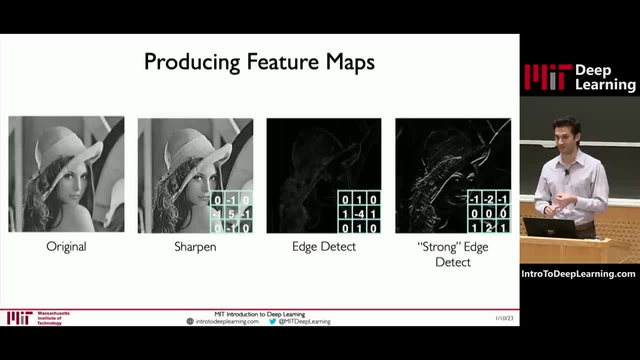 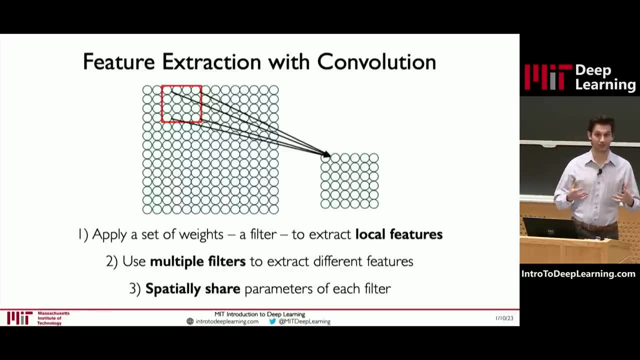 extract edges. We can do stronger edge detection by again modifying the weights in all of those filters. So I hope now that all of you can kind of appreciate the power of you know. number one is these filtering operations and how we can define them. you know, mathematically, in the form: 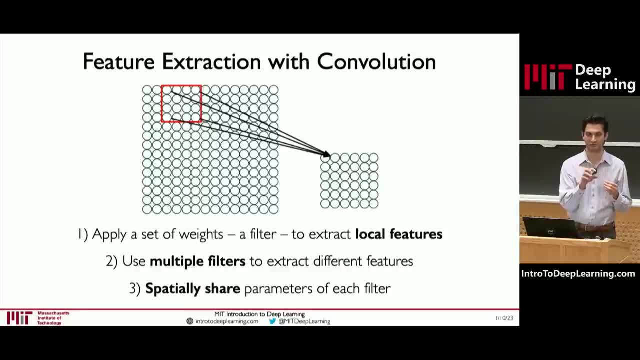 of these smaller patch-based operations and matrices that we can then slide over an image. And these concepts are so powerful because, number one, they preserve the spatial information of our original input while still performing this feature extraction. Now you can think of: 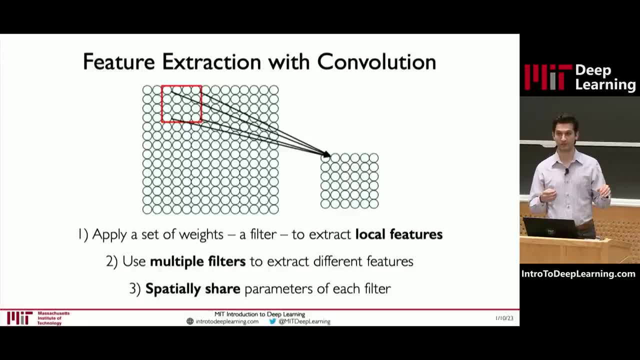 instead of defining those filters, like we said on the previous slide, what if we tried to learn them And remember again that those filters are kind of proxies for important patterns in our data? So our neural network could try to learn those elements of those small patch filters as weights in the neural network And learning those. 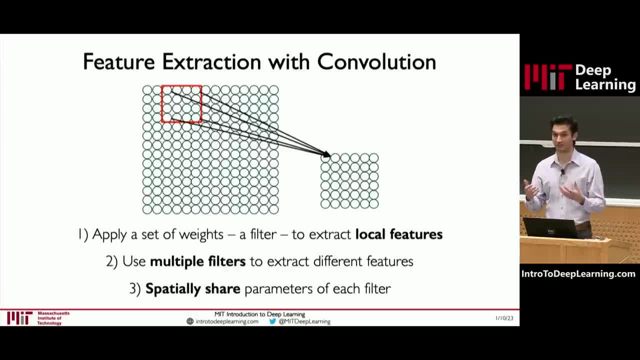 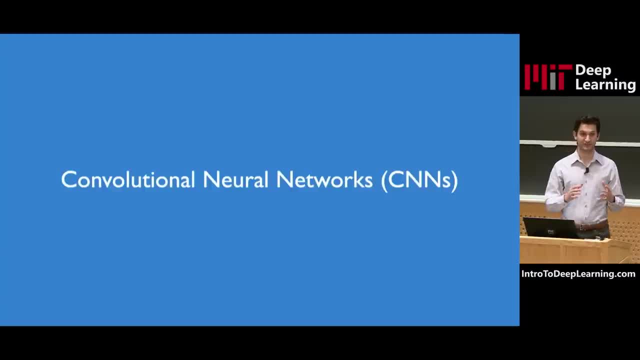 would essentially equate to picking up and learning the patterns that define one class versus another class. And now that we've gotten this operation and this understanding under our belt, we can take this one step further. right, We can take this singular convolution operation. 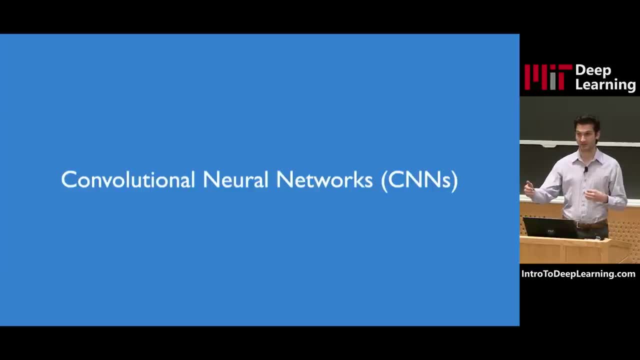 and start to think about how we can build entire layers, convolutional layers, out of this operation, So that we can start to even imagine convolutional networks and neural networks. And first we'll take a look at- you know what are called. well, what you ultimately create by creating convolutional 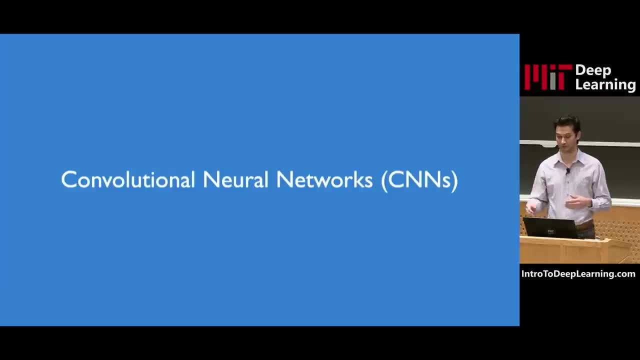 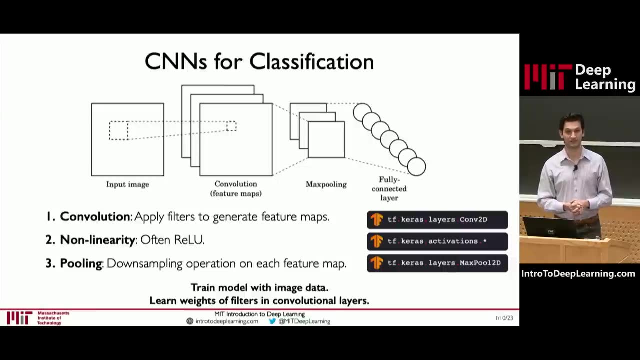 layers and convolutional networks is what's called a CNN, a convolutional neural network, And that's going to be the core architecture of today's class. So let's consider a very simple CNN that was designed for image classification. The task here again is to learn the features directly from the 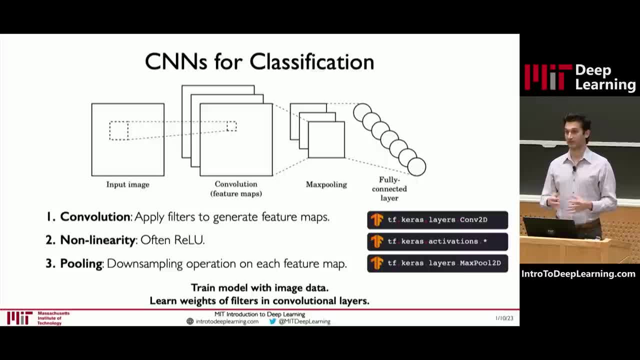 raw data And use these learned features for classification towards some task of object detection that we want to perform. Now there are three main operations to a CNN And we'll go through them step by step here but then go deeper into each of them in the remainder of this class. 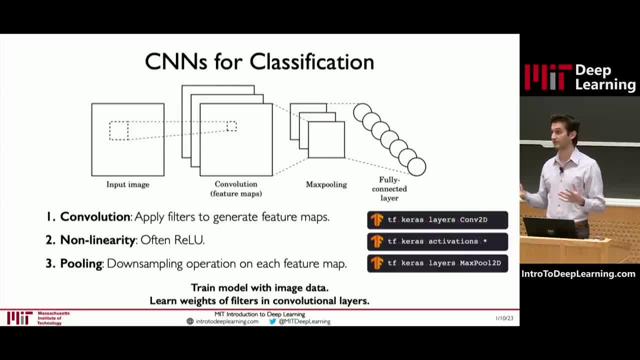 So the first step is convolutions, which we've already seen a lot of in today's class. already, Convolutions are used to generate these feature maps, So they take as input both the previous image as well as some filter that they want to detect, and they output a feature map of how this filter is. 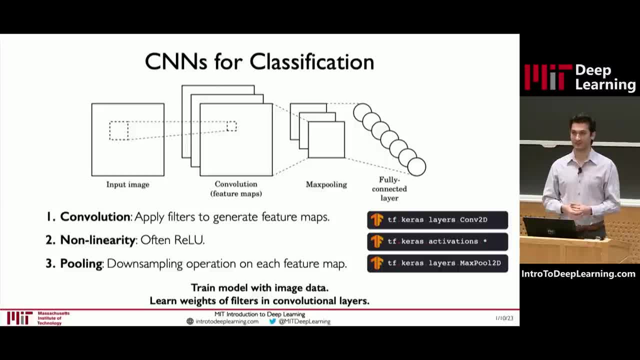 related to the original image. The second step is, like yesterday, applying a non-linearity to the result of these feature maps. That injects some non-linear activations to our neural networks. allows it to deal with non-linear data. Third step is pooling, which is essentially a downsampling. 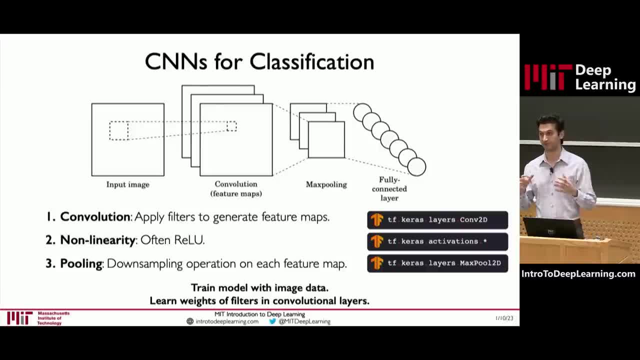 operation to allow our images or allow our networks to deal with larger and more complex features. So this is a well-designed solution for the neural network. So we can see that these features can be used to create larger and larger scale images by progressively downscaling their size so that our filters can progressively grow in receptive field. 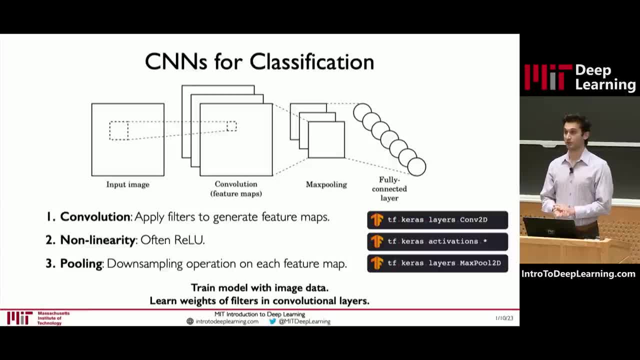 And finally, feeding all of these resulting features to some neural network to infer the class scores. Now, by the time that we get to this fully connected layer, remember that we've already extracted our features And essentially, you can think of this no longer being a two-dimensional image. 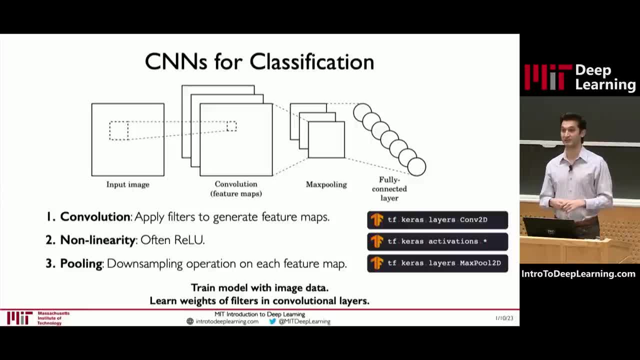 use the methods that we learned about in lecture one to directly take those learned features that the neural network has detected and infer based on those learned features and based on, if they were detected or if they were not, what class we're in. So now let's basically just go through. 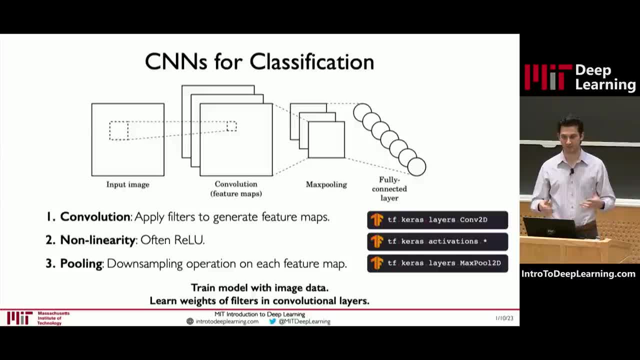 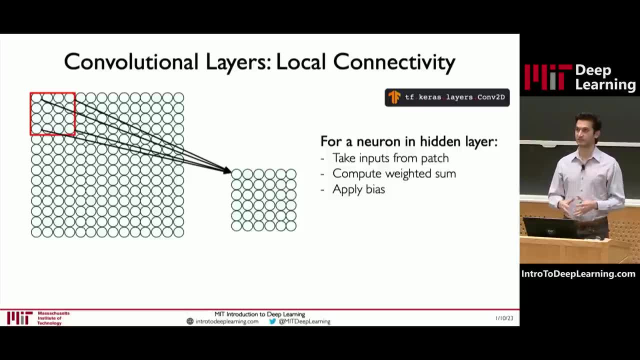 each of these operations one by one in a bit more detail and see how we could even build up this very basic architecture of a CNN. So first let's go back and consider one more time the convolution operation. that's a central core to the CNN. 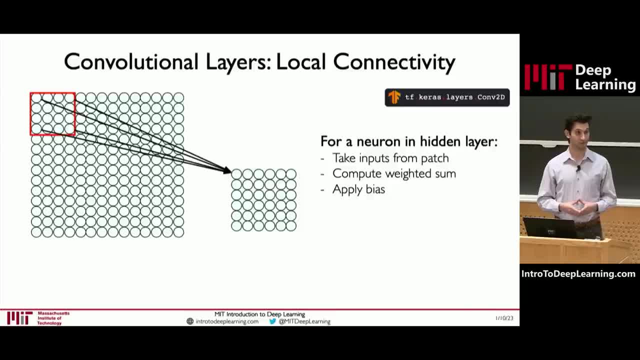 And, as before, each neuron in this hidden layer is going to be computed as a weighted sum of its inputs. applying a bias and activating with a nonlinearity Should sound very similar to lecture one in yesterday's class, but except now. 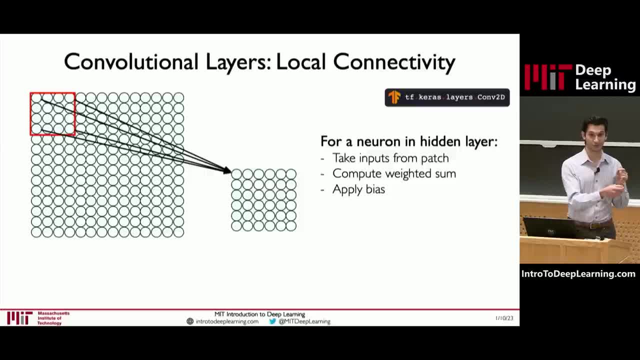 when we're going to do that first step, instead of just doing a dot product with our weights, we're going to apply a convolution with our weights which is simply that element-wise multiplication and addition right, and that sliding operation. Now, what's really special here? 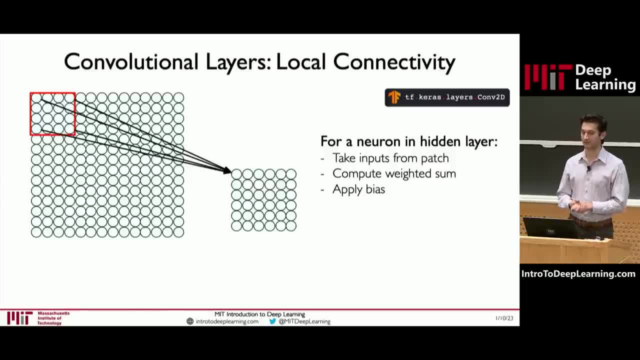 and what I really want to stress is the local connectivity. Every single neuron in this hidden layer only sees a certain patch of inputs in its previous layer. So if I point at just this one neuron in the output layer, this neuron only sees the inputs at this red square. 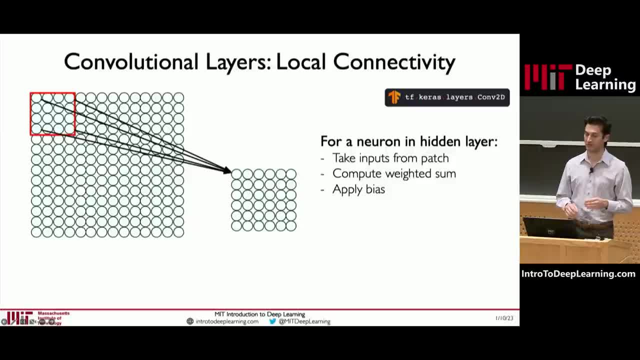 It doesn't see any of the other inputs in the rest of the image And that's really important to be able to scale these models to very large-scale images. Now you can imagine that as you go deeper and deeper into your network, eventually because the next layer 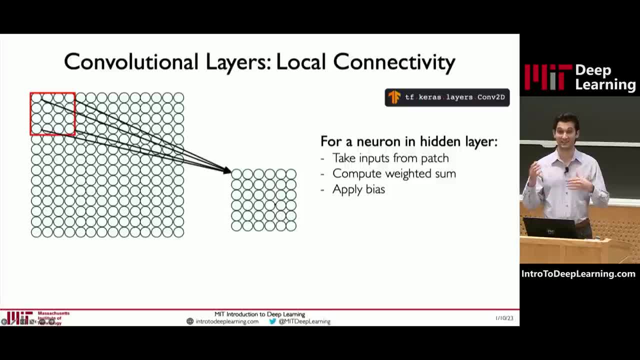 you're going to attend to a larger patch, right, And that will include data from not only this red square, but effectively a much larger red square that you could imagine there. Now let's define this actual computation that's going on For a neuron in a hidden layer. its inputs are those neurons. 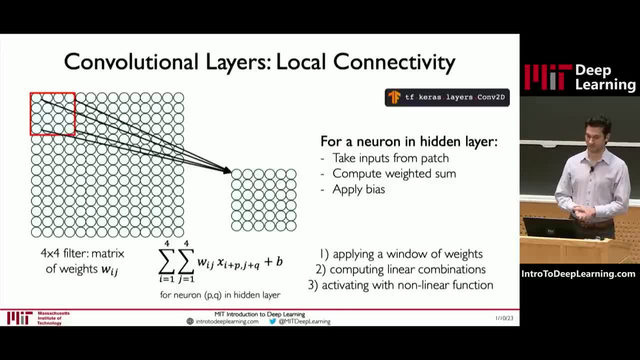 right. These are the neurons that fell within its patch in the previous layer. We can apply this matrix of weights- here denoted as a 4 by 4 filter that you can see on the left-hand side, And in this case we do an element-wise multiplication. 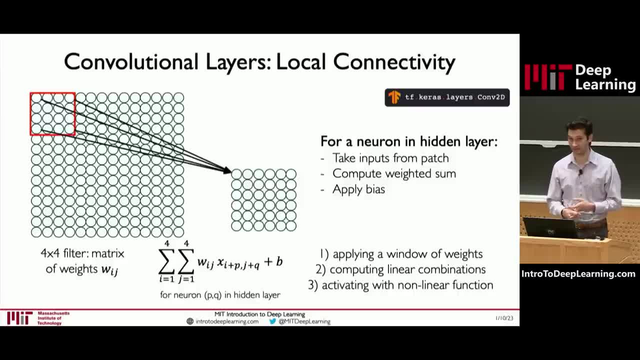 We add the outputs, we apply a bias and we add that non-linearity. right, That's the core steps that we take in really all of these neural networks that you're learning about in today's and this week's class. to be honest, 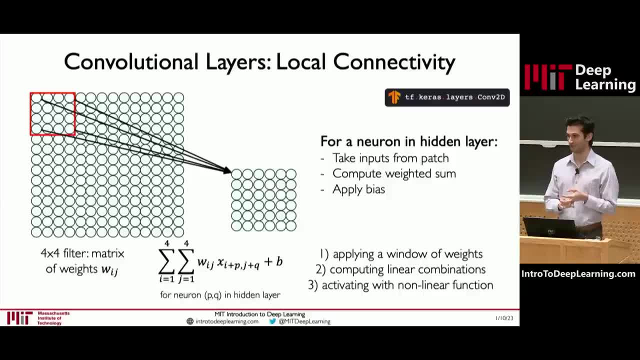 Now remember that this element-wise multiplication and addition operation, that sliding operation that's called convolution and that's the basis of these layers. So that defines how neurons in convolutional layers are connected, how they're mathematically formulated, But within a single convolutional layer. 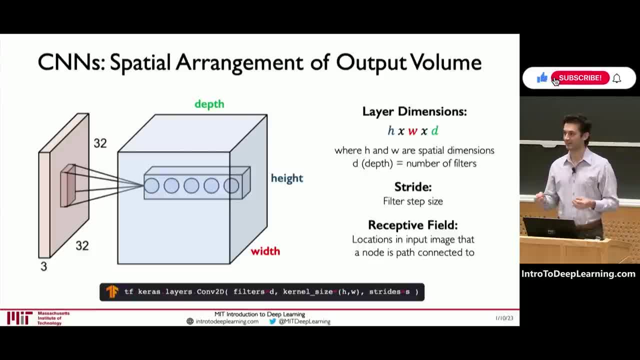 it's also really important to understand that a single layer could actually try to detect multiple sets of filters, right? Maybe you want to detect in one image multiple features, not just one feature. But if you were detecting multiple features, if you were detecting faces, you don't only want to detect eyes. 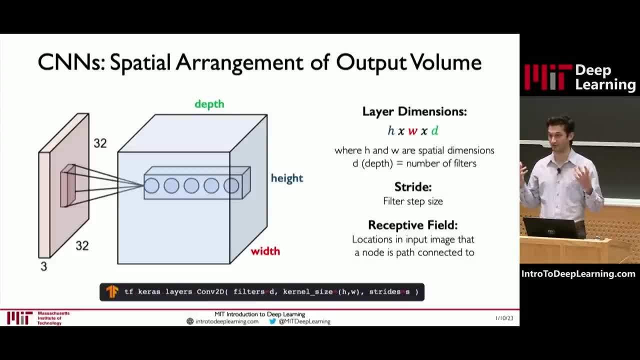 You want to detect eyes, noses, mouths, ears, right- All of those things are critical patterns that define a face and can help you classify a face. So what we need to think of is actually convolution operations that can output a volume of different images, right? 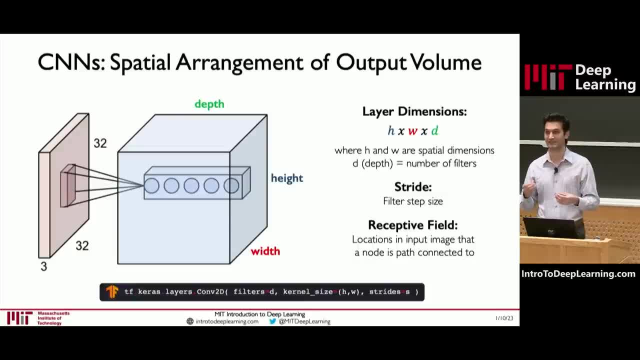 Every slice of this volume effectively denotes a different filter that can be identified in our original input, And each of those filters is going to basically correspond to a specific pattern or feature in our image as well. Think of the connections in these neurons in terms of their receptive field. once again, right. 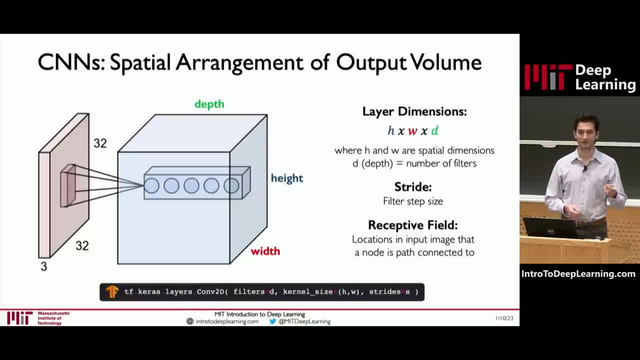 The locations within the input of that node that they were connected to in the previous layer. These parameters really define what I like to think of as the spatial arrangement of information that propagates throughout the network and throughout the convolutional layers, in particular, Woo. 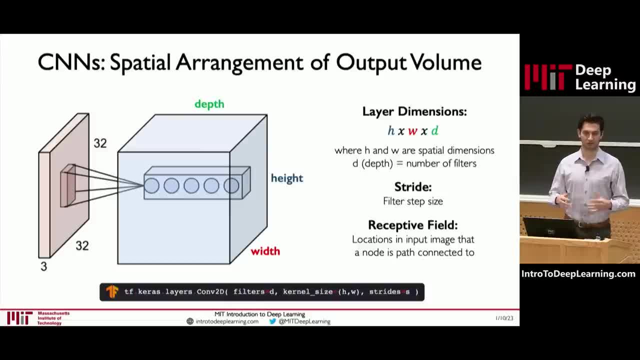 Now I think, just to summarize what we've seen and how connections in these types of neural networks are defined, and let's say how the output of a convolutional network is a volume- We are well on our way to really understanding convolutional neural networks and defining them right. 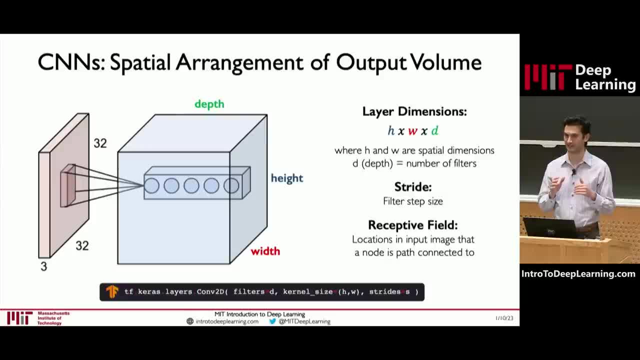 That's the. what we just covered is really the main component of CNN's right. That's the convolutional operation that defines these convolutional layers. The remaining steps are very critical as well, but I want to maybe pause for a second and make. 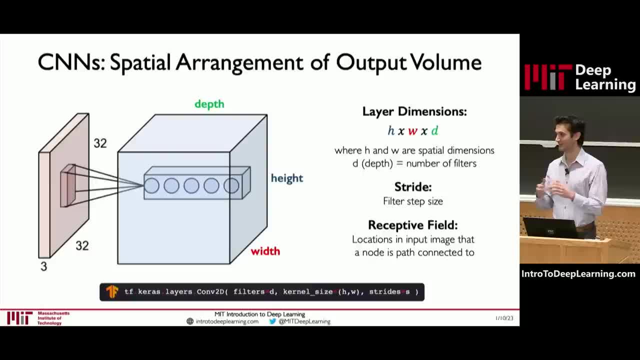 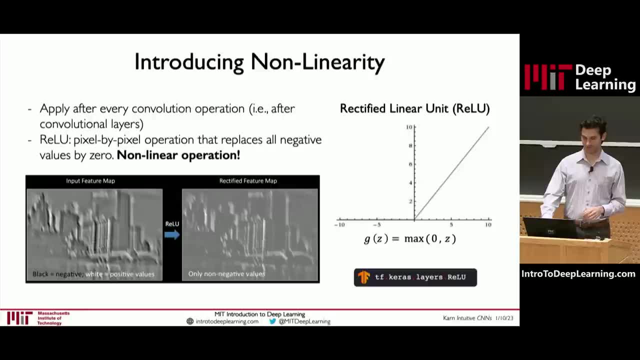 sure that everyone's on the same page with the convolutional operation and the definition of convolutional layers- Awesome, Okay. So the next step here is to take those resulting feature maps that our convolutional layers extract and apply a non-linearity to the output volume. 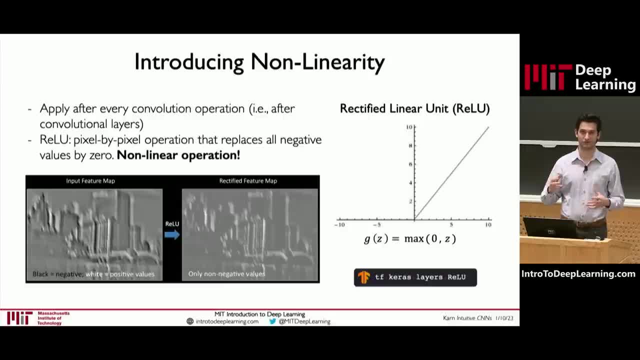 of the convolutional layer. So, as we discussed in the first lecture, applying these non-linearities is really critical because it allows us to deal with non-linear data and because image data in particular is extremely non-linear. that's a critical component of what makes convolutional neural networks actually operational in practice. 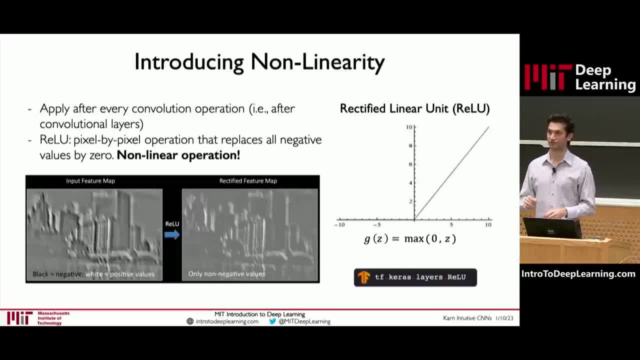 In particular for convolutional neural networks. the activation function that is really really common for these models is the ReLU activation function. We talked a little bit about this in lecture one. We talked a little bit about this in lecture two, but I want to. 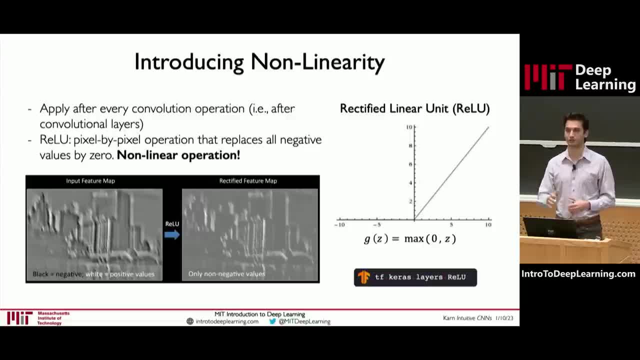 talk a little bit about this in lecture one and two yesterday, The ReLU activation function. you can see it on the right-hand side. Think of this function as a pixel-by-pixel operation that replaces basically all negative values with zero. It keeps all positive values the same. It's the identity function when a value is positive, but when it's negative it basically squashes everything back up to zero. Think of this almost as a thresholding function. right Thresholds is everything at zero. Anything less than zero comes back up to zero. So negative values here indicate. 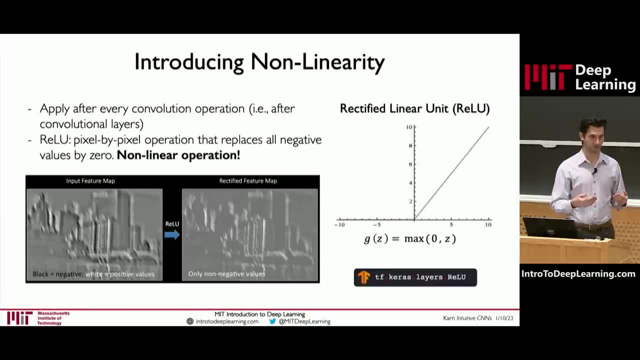 basically a negative detection in convolution that you may want to just say was no detection right, And you can think of that as kind of an intuitive mechanism for understanding why the ReLU activation function is so popular in convolutional neural networks. The other popular belief is that ReLU activation functions well. it's not a belief. They are extremely easy to compute and they're very easy and computationally efficient. Their gradients are very cleanly defined. They're constants, except for a piecewise. 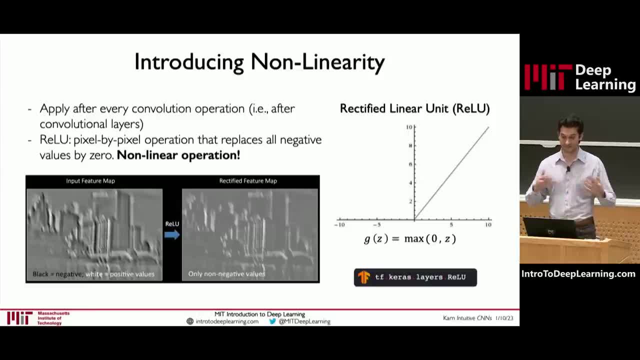 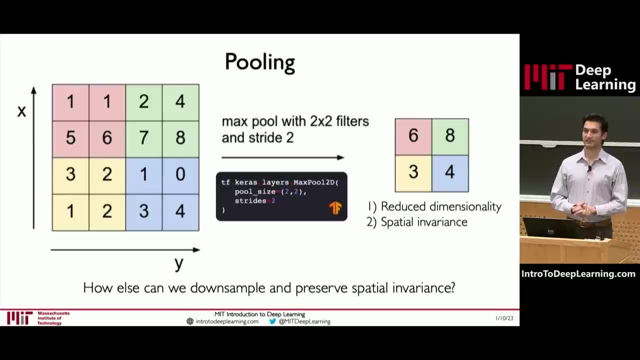 non-linearity, So that makes them very popular for these domains. Now the next key operation in a CNN is that of pooling. Now, pooling is an operation that is at its core. it serves one purpose and that is to reduce the dimensionality of the image progressively as you go deeper and deeper through your convolutional layers. Now you can really start to reason about this is that when you decrease the dimensionality of your feature, you increase the dimensionality of your feature and you increase the dimensionality of your feature. So that's a very popular belief. 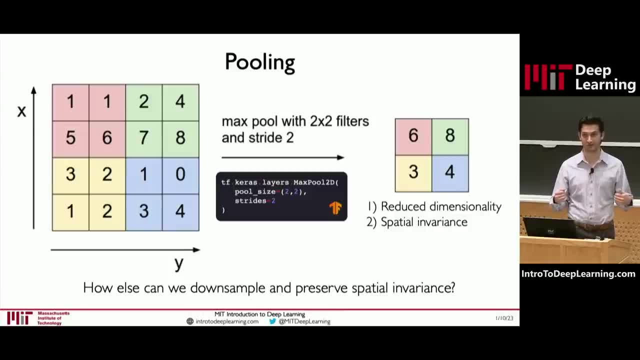 features. you're effectively increasing the dimensionality of your filters right Now, because every filter that you slide over, a smaller image is capturing a larger receptive field that occurred previously in that network. So a very common technique for pooling is what's called. 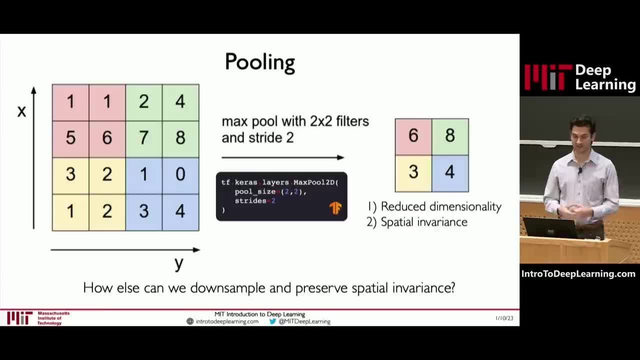 maximum pooling, or max pooling for short. Max pooling is exactly. you know what it sounds like. So it basically operates with these small patches, again that slide over an image, But instead of doing this convolution operation, what these patches will do is simply take the maximum of. 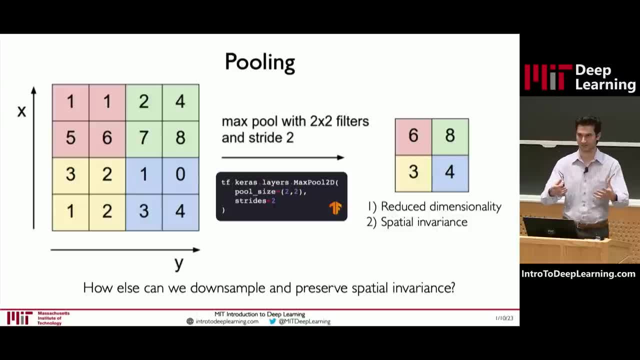 that patch location. So think of this as kind of activating the maximum value that comes from that location and propagating only the maximums. I encourage all of you actually to think of, maybe brainstorm, other ways that we could perform even better pooling operations than max pooling. 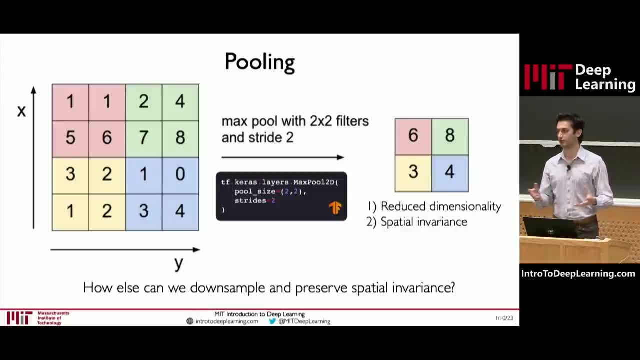 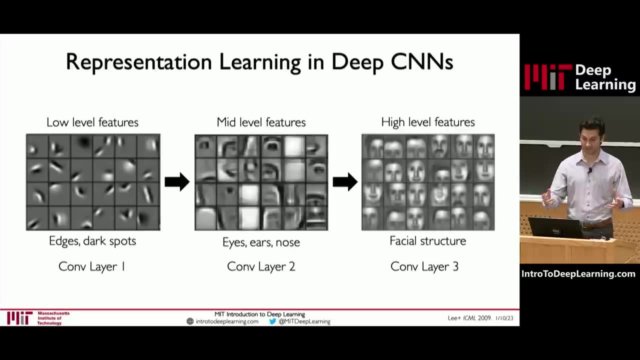 There are many common ways, but you could think of some. for example are mean pooling or average pooling. right, Maybe you don't want to just take the maximum. You could collapse basically the average of all of these pixels into your single value in the result. But these are the key operations of convolutional neural networks at 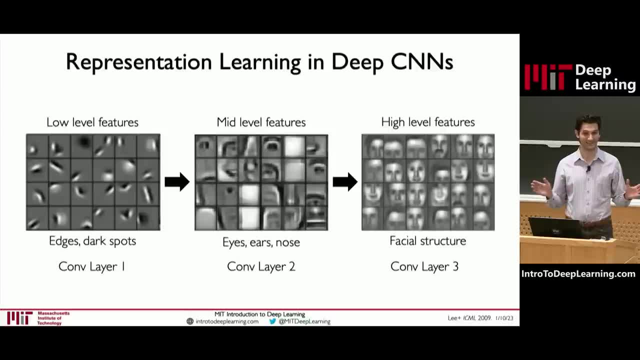 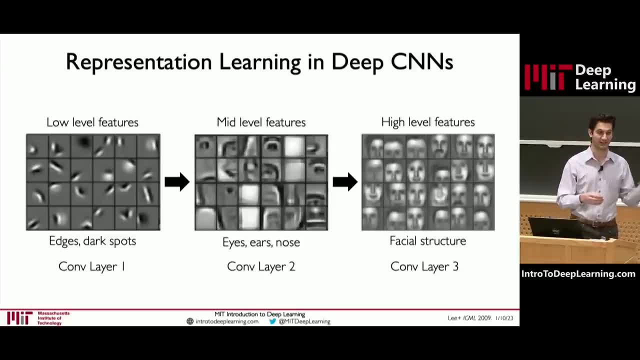 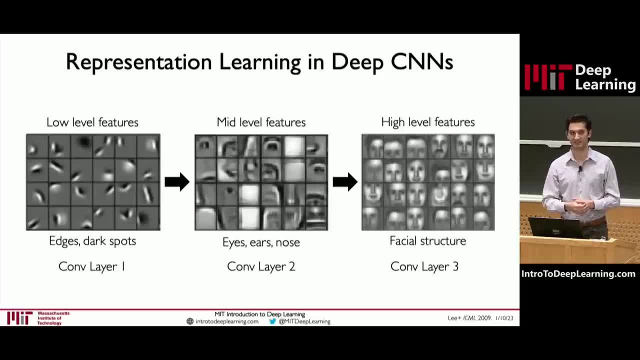 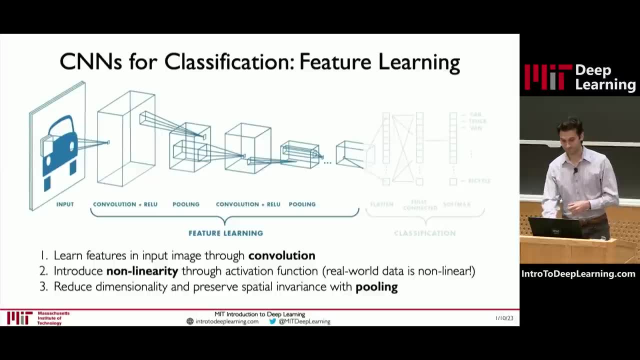 decompositions of features by progressively stacking and stacking these filters on top of each other. Each filter could then use all of the previous filters that it had learned. So a CNN built for image classification can be really broken down into two parts. First is the feature learning pipeline which we learn. 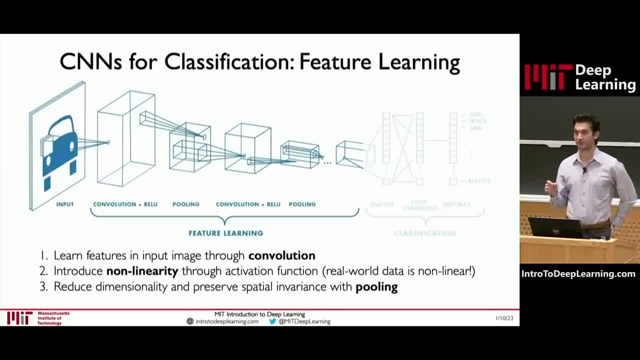 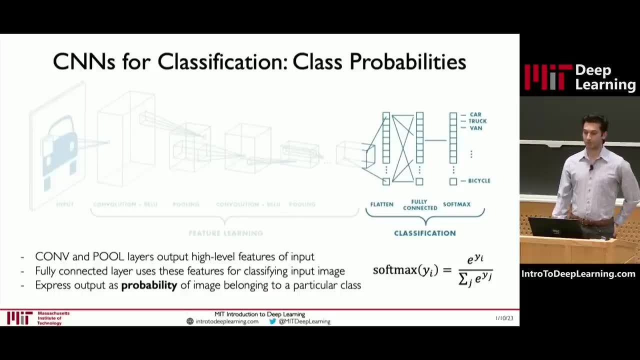 the features that we want to detect. and then the second part is actually detecting those features and doing the classification. Now the convolutional and pooling layers output from the first part of that model. the goal of those convolutional and pooling layers is to output the high level features. 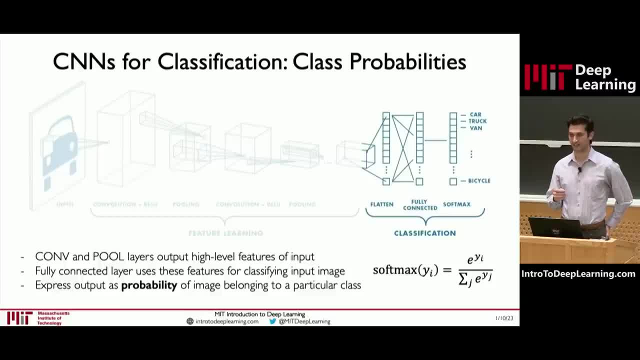 that are extracted from our input, but the next step is to actually use those features and detect their presence in order to classify the image, So we can feed these outputted features into the fully connected layers that we learned about in lecture one, because these are now just a. 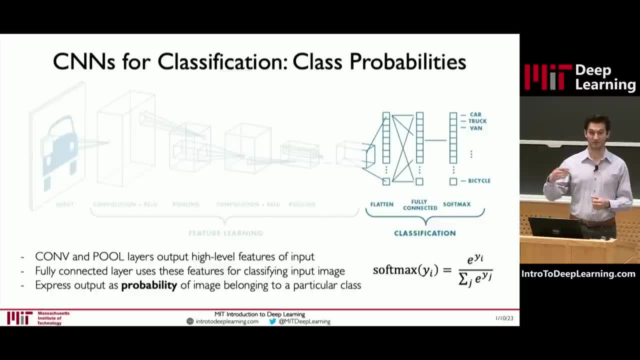 one-dimensional array of features and we can use those to detect. you know what class we're in, and we can do this by using a function called a softmax function. You can think of a softmax function as simply a normalizing function whose output represents that of a categorical probability. 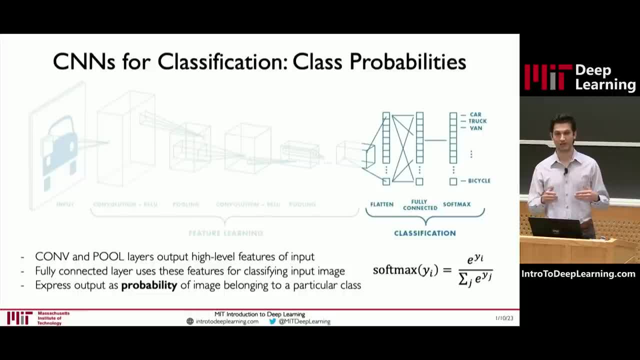 distribution. So another way to think of this is basically: if you have an array of numbers, you want to collapse, and those numbers could take any real number form, you want to collapse that into some probability distribution. Probability distribution has several properties, namely that all of its values have to. 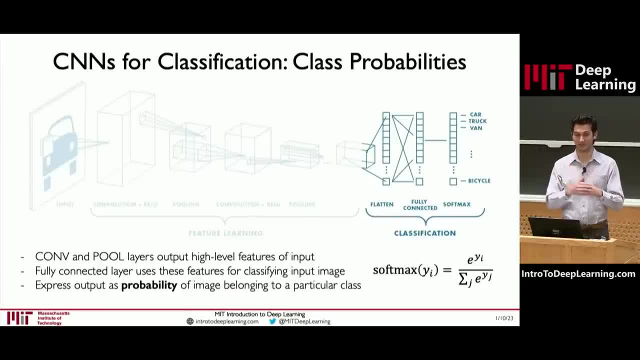 sum to one. It always has to be between zero and one as well. So maintaining those two properties is what a softmax operation does. You can see its equation right here. It effectively just makes everything positive, and then it normalizes the result across each other, and that may. 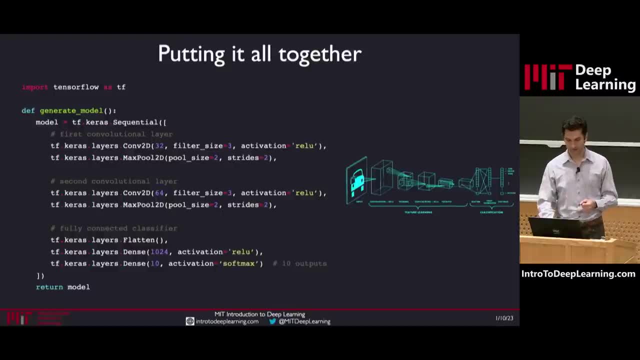 contain those two properties that I just mentioned. Great. So let's put all of this together and actually see how we could program our first convolutional neural network, end to end, entirely from scratch. So let's start by firstly defining our feature extraction head, which starts with a convolutional layer and here 32 filters, or 32. 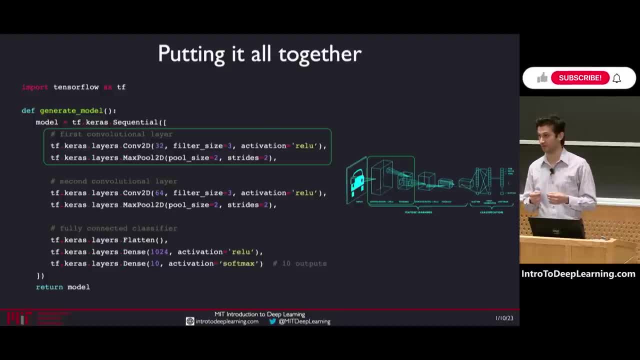 features. You can imagine that this first layer, the result of this first layer, is to learn not one filter, not one pattern. It's not just our image, but 32 patterns. OK, So those 32 results are going to then be passed to a 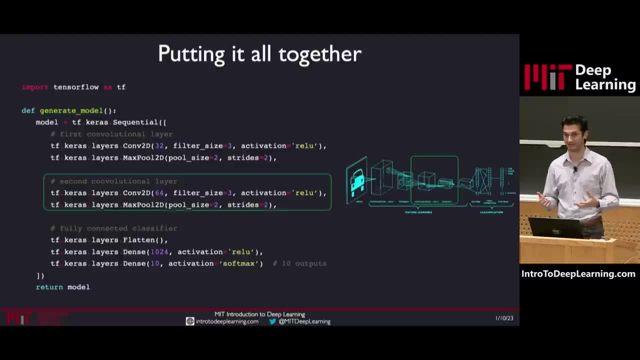 pooling layer and then passed on to the next set of convolutional operations. The next set of convolutional operations now will contain 64 features, will keep progressively growing and expanding our set of patterns that we're identifying in this image. Next we can finally flatten those resulting features that we've identified and feed all of this through our 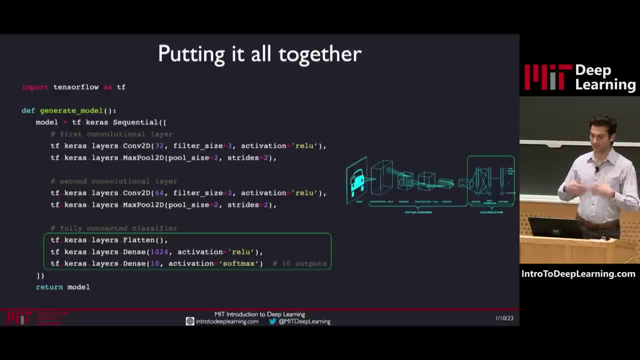 identity. So let's say we have a bunch of layers in our image, So we have our dense layers are fully connected layers that we learned about in lecture one. These will allow us to predict those final- let's say 10 classes. if we have 10 different final possible classes in our image, This layer will account for that. 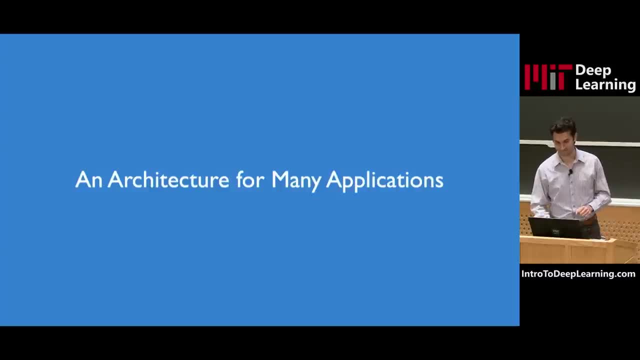 and allow us to output, using softmax, the probability distribution across those 10 classes. So so far we've talked about, right, how we can, let's say, use CNN's to perform image classification tasks, And what we've learned in this class, especially towards the end, is that this same architecture and same building blocks that we've talked about so far are extensible, and they extend to so many different applications and model types that we can imagine. 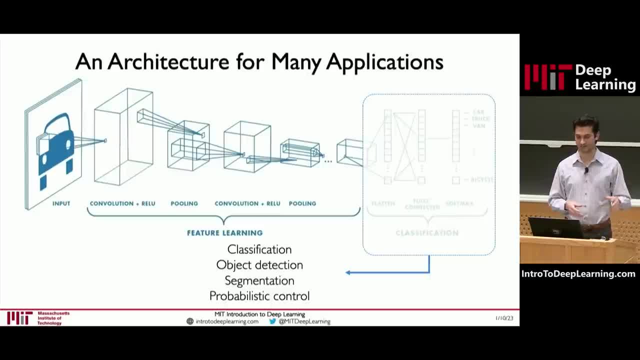 So, for example, when we considered the CNN for classification, we saw that it really had two parts right, the first part being feature extraction, learning what features to look for, and the second part being the classification, the detection of those features. Now, what makes a convolutional neural network really, really powerful is exactly the observation that the feature learning part, this first part of the neural network, is extremely flexible. 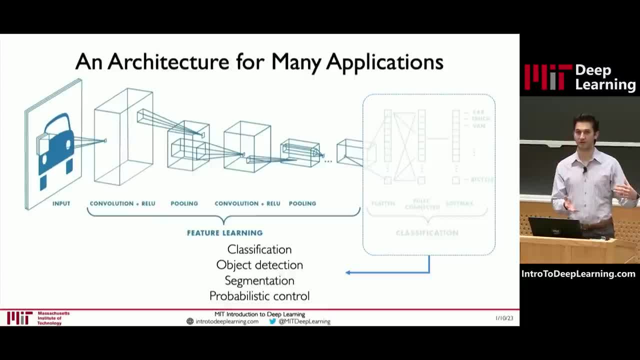 You can take that first part of the neural network, chop off what comes after it and put a bunch of different heads into the part that comes after it. The goal of the first part is to extract those features. What you do with the features is entirely up to you. 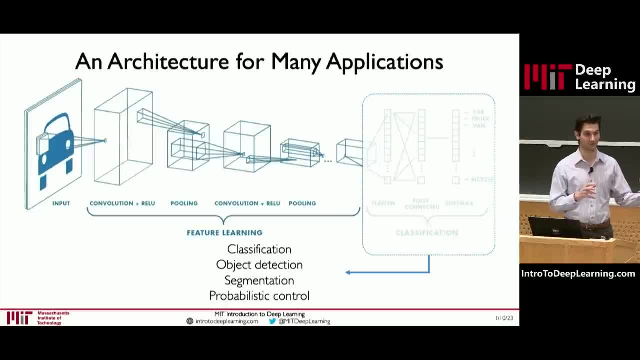 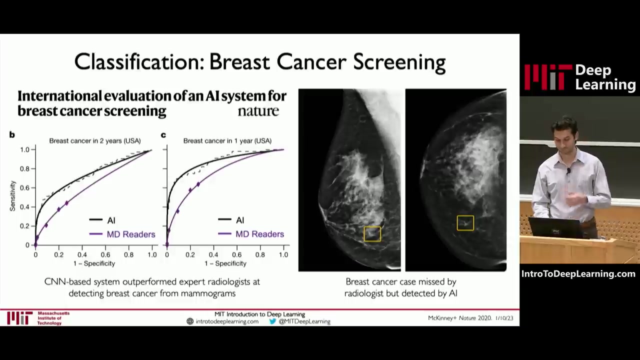 But you can step back and look at it. You can still leverage the flexibility and the power of the first part to learn all of those core features. So, for example, that portion will look for you know all of the different image classification domains, that future portion, after you've extracted the features. or we could also introduce new architectures that take those features and maybe perform tasks like segmentation or image captioning, like we saw in yesterday's lecture. 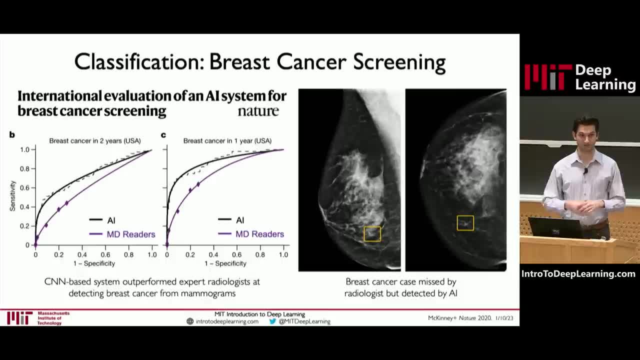 So in the case of classification, for example- just to tie up the classification story- There's a significant impact in domains like health care, medical decision making, where deep learning models are being applied to the analysis of medical scans across a whole host of different medical imagery. 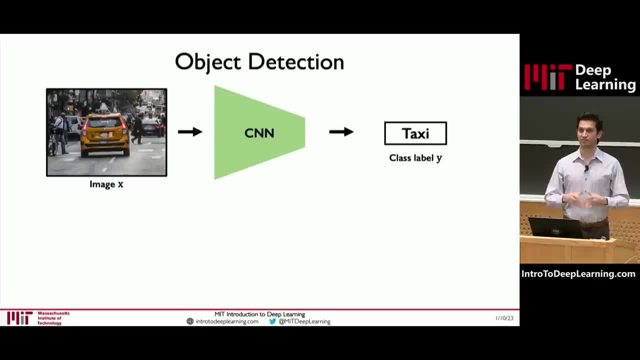 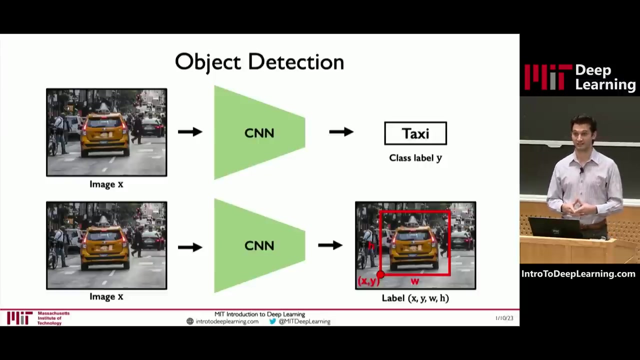 Now, classification tells us basically a discrete prediction of what our image contains, But we can actually go much deeper into this problem as well. So, for example, imagine that we're not trying to only identify that this image Is an image of a taxi, which you can see here, but also, more importantly maybe, we want our neural network to tell us not only that this is a taxi, but identify and draw a specific bounding box over this location of the taxi. 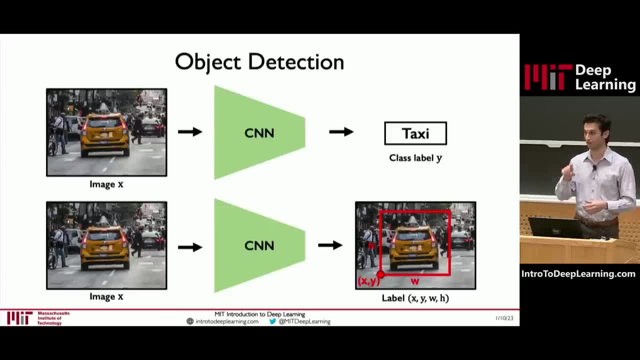 So this is kind of a two phase problem. Number one is that we need to draw a box, and number two is we need to classify what was in that box Right. So it's both a regression problem: Where is the box Right? 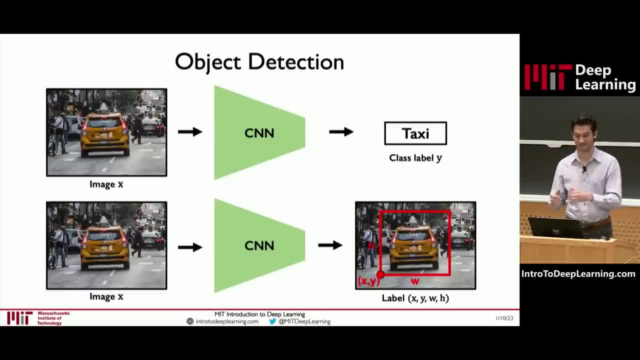 What is this problem, as well as a classification problem, is: what is in that box? Now, that's a much, much harder problem than what we've covered so far in the lecture today, because potentially there are many objects in our scene, not just one object, Right, 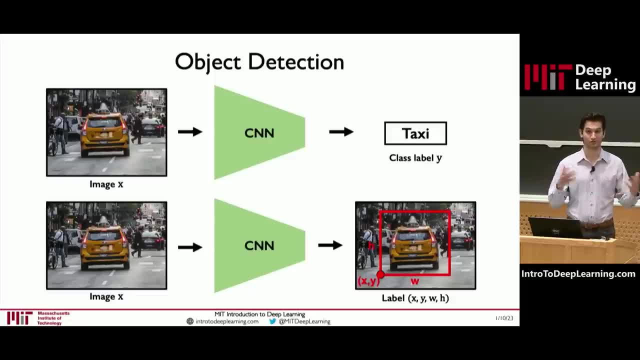 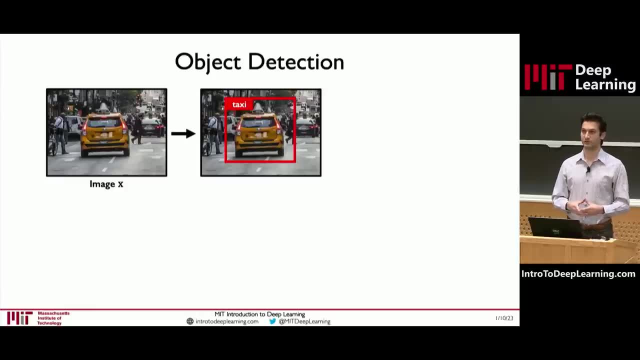 So we have to account for this fact that maybe our scene could contain arbitrarily many objects. Now our network needs to be flexible to that degree. Right, It needs to be able to infer a dynamic number of objects In the scene. And if the scene is only of a taxi, then it should only output, you know that, one bounding box. 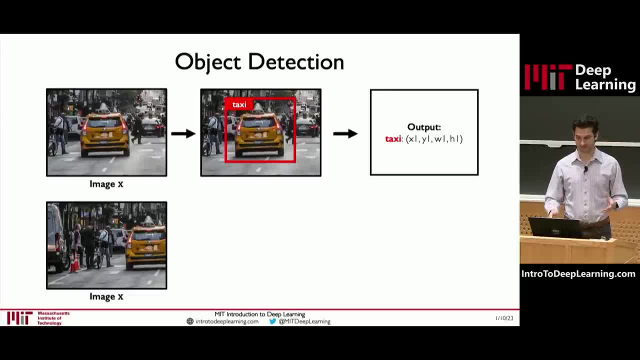 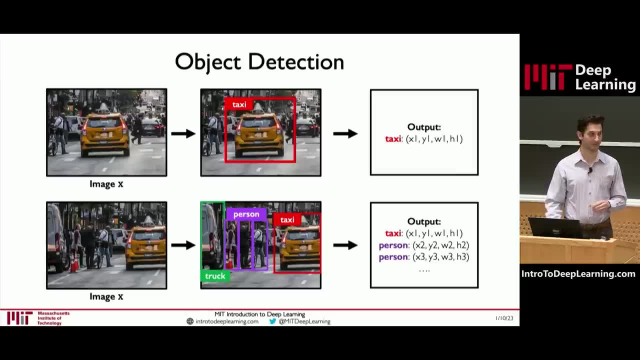 But, on the other hand, if the image has many objects right, potentially even of different classes, we need a model that can draw a bounding box for each of these different examples, as well as associate their predicted classification labels to each one independently. Now this is actually quite complicated in practice. 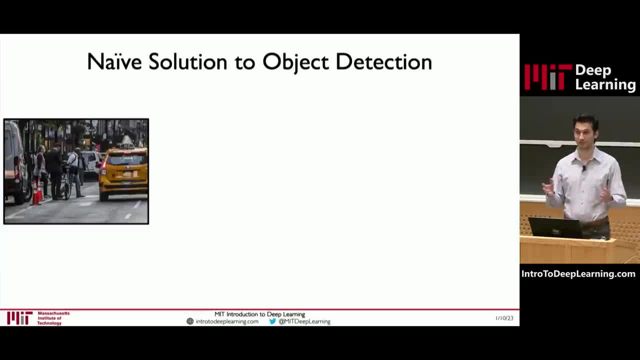 Because those boxes Can be anywhere in the image Right. There's no constraints on where the boxes can be And they can also be of different sizes. They can be also different ratios, Right. Some can be tall, some can be wide. 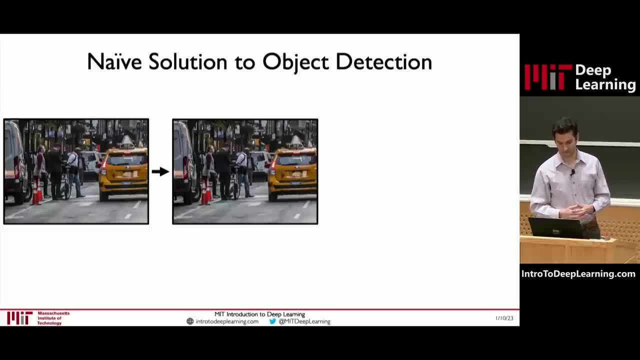 Let's consider a very naive way of doing this. First, let's take our image and start by placing a random box somewhere on that image. For example, we just pick a random location, a random size. We'll place a box right there. This box, like I said, has a random location, random size. 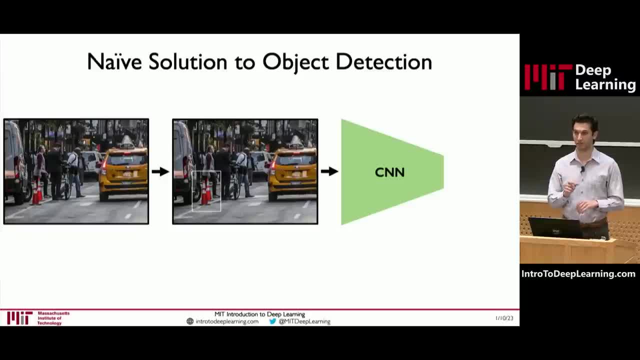 Then we can take that box and only feed that random box through our convolutional neural network, which is trained to do classification, just classification, And this neural network can detect. well, number one: is there a class of object in that box or not? And if so, what class is it? 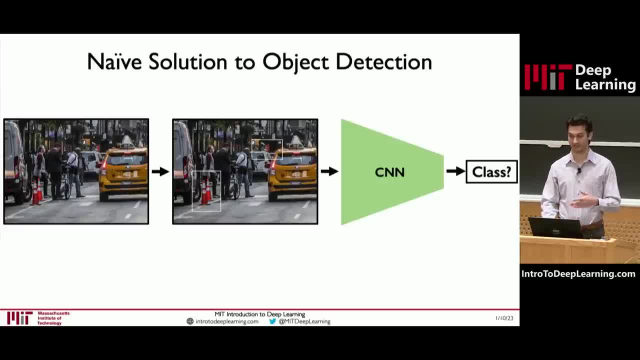 And then what we can do is we could just keep repeating this process over and over again for all of these random boxes in our image. You know many, many instances of random boxes. We keep sampling a new box, Feed it through our convolutional neural network and ask this question: what was in the box? 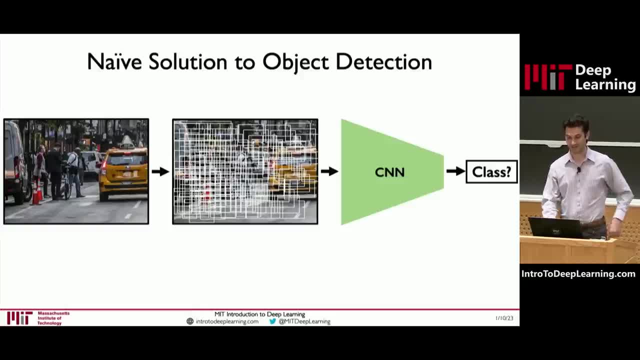 If there was something in there, then what? what is it Right? And we keep moving on until we kind of have exhausted all of the boxes in the image. But the problem here is that there are just way too many potential inputs that we would have to deal with. 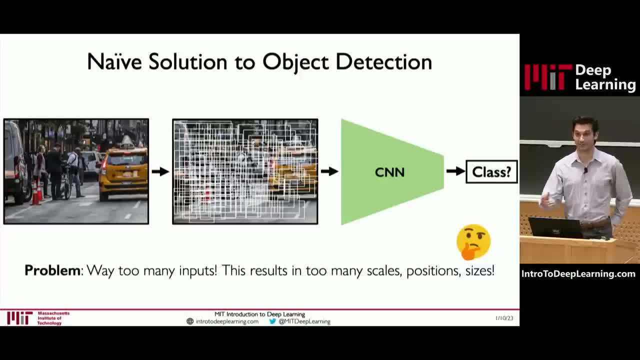 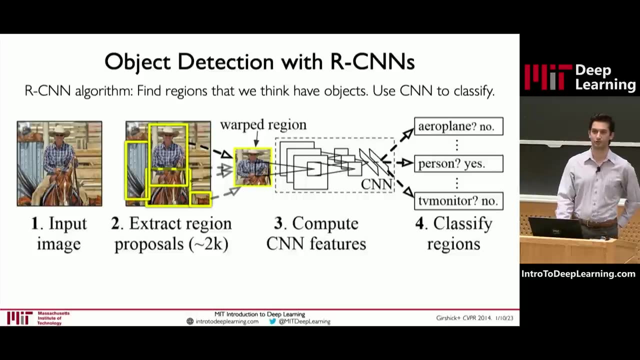 This would be totally impractical to run in a real time system. For example, with today's compute it results in way too many scales, especially for the types of resolutions of images that we deal with today, Right? So instead of picking random boxes, let's try and use a very simple heuristic right to identify maybe some places with lots of variability in the image where there is high likelihood of having an object might be present. 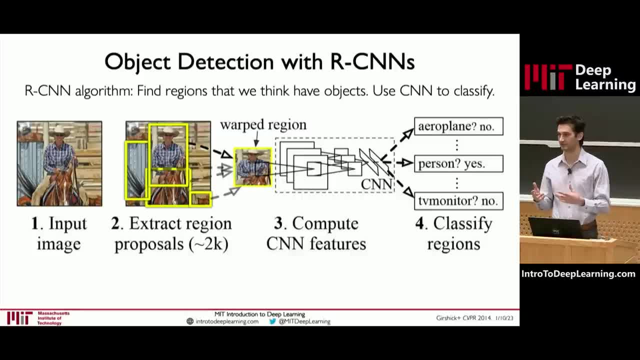 Right, These might have meaningful insights or meaningful objects that could be available in our image and we can use those to basically just feed in those high attention locations to our convolutional neural network And then we can basically speed up that first part of the pipeline a lot, because now we're not just picking random boxes. 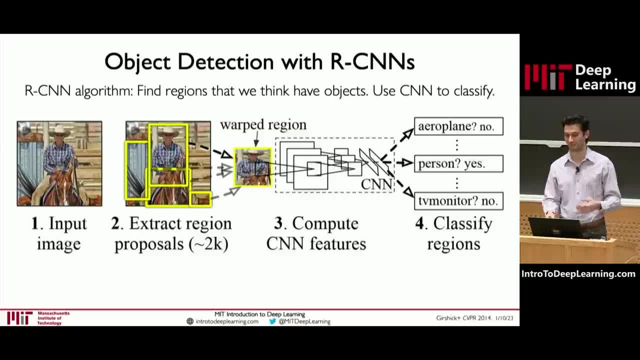 Maybe we use like some simple heuristic to identify where interesting parts of the image might be, But still this is actually very slow in practice. We have to feed in each region independently to the model And plus it's very brittle because ultimately the part of the model that is looking at where potential objects might be is detached from the part that's doing the detection of those objects. 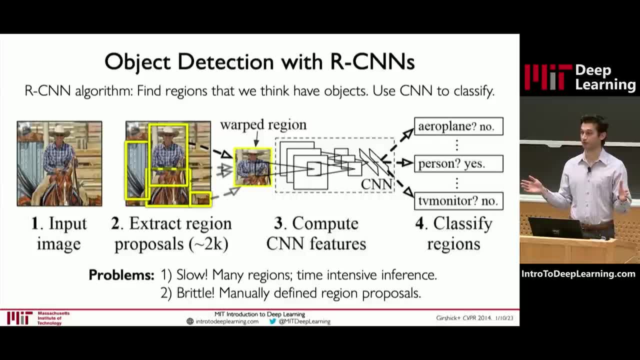 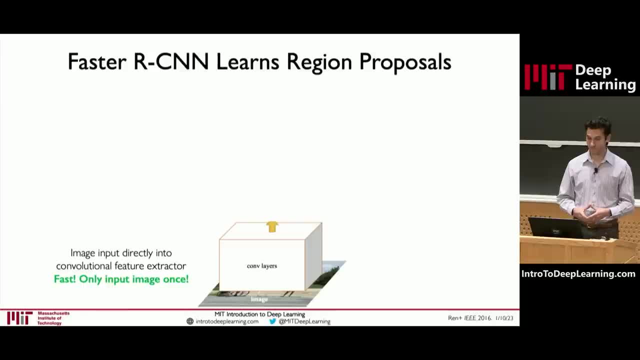 Ideally we want one model that is able to, both you know, figure out where to attend to and do that classification afterwards. So there have been many variants that have been proposed in this field of object detection, But I want to, just for the purpose of today's class, introduce you to one of the most popular ones. 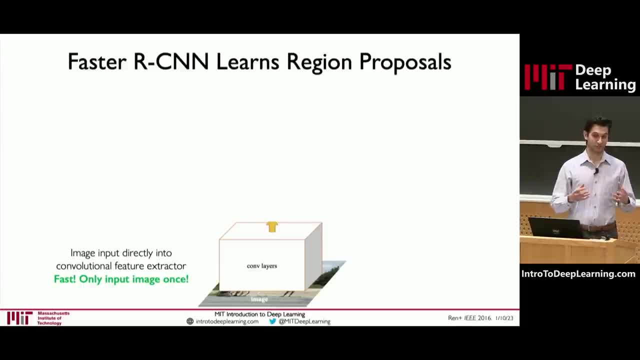 Now this is a point, or this is a model called RCNN, or faster RCNN, Which actually attempts to learn Not only how to classify these boxes, but learns how to propose those where those boxes might be in the first place, so that you could learn how to feed or where to feed into the downstream neural network. 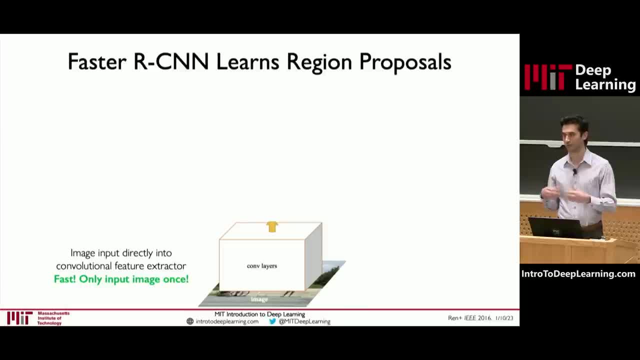 Now this means that we can feed in the image to what are called these region proposal networks. The goal of these networks is to propose certain regions in the image that you should attend to and then feed just those regions into the downstream CNNs. So 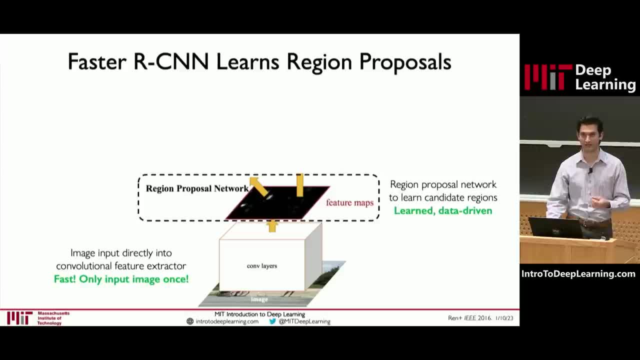 The goal here is to directly try to learn or extract all of those key regions and process them through the later part of the model. Each of these regions are processed with their own independent feature extractors and then a classifier can be used to aggregate them all and perform feature detection as well as object detection. 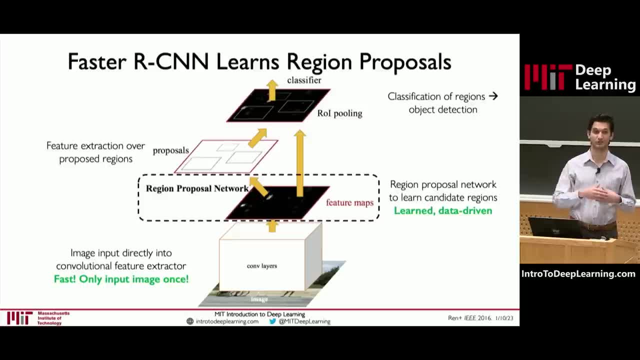 Now, the beautiful thing about this is that this requires only a single pass through the network, So it's extraordinarily fast, It can easily run in real time, And it's very commonly used in many industry applications as well. Even it can even run on your smartphone. 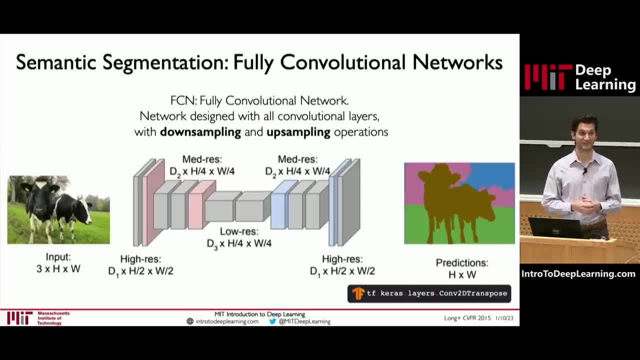 So in classification, we just saw how we can predict, you know, not only a single image per, or sorry, a single object per image. We saw an object detection potentially inferring multiple objects with bounding boxes in your image. There's also one more type of task which I want to point out, which is called segmentation. 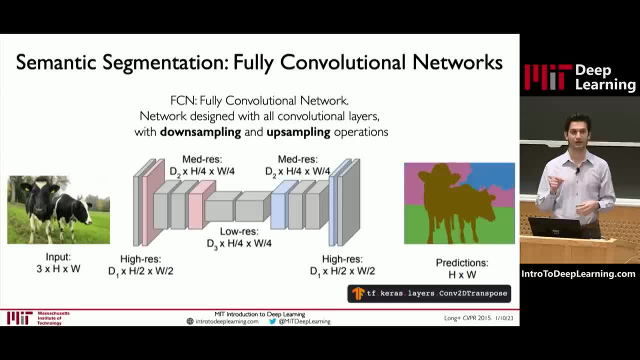 Segmentation is the task of classification, but now done at every single pixel. This takes the idea of object detection, which bounding boxes, to the extreme. Now, instead of drawing boxes, we're not even going to consider boxes- We're going to learn how to classify every single pixel in this image in isolation. 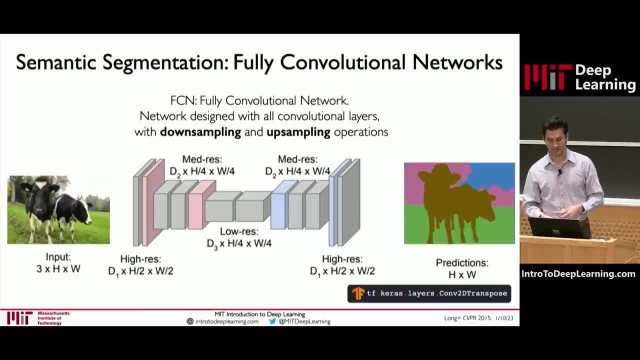 Right. So it's a huge number of classifications that we're going to do, and we'll do this Well, first let me show this example. So, on the left hand side, what this looks like is your feeding image. The goal of the right hand side is to learn for every pixel. in the left hand side, 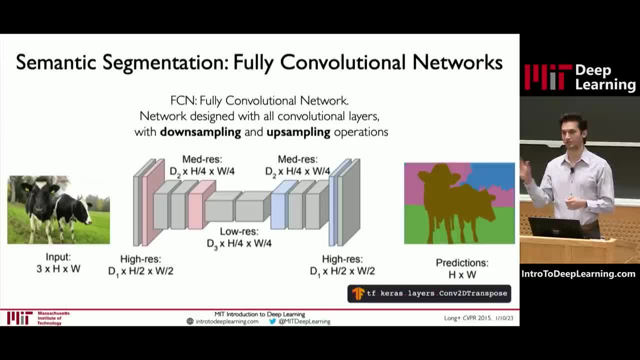 What was the class of that pixel, Right? So this is kind of in contrast to just determining, you know, boxes over our image. Now we're looking at every pixel in isolation and you can see, for example, you know this: pixels of the cow are clearly differentiated from the pixels of the sky or the pixels of the grass. 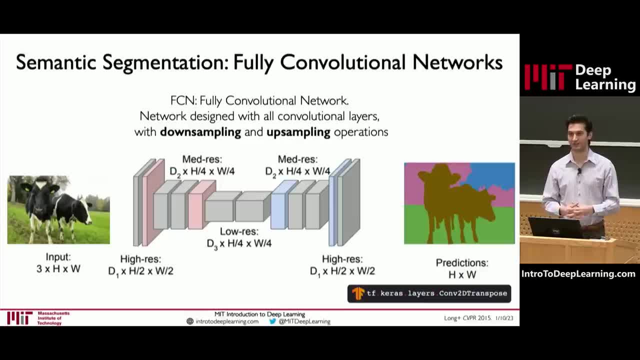 Right And that's a create a key, critical component Of semantic segmentation networks. The output here is created by again using these convolutional operations, followed by pooling operations which learn an encoder which you can think of on the left hand side. These are learning the features from our RGB image, learning how to put them into a space so that it can reconstruct into a new space of semantic labels. 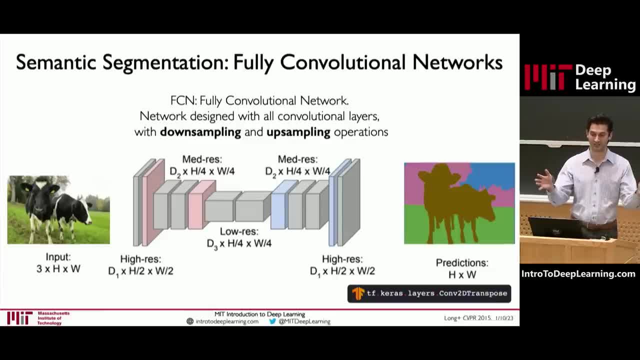 So you can imagine kind of a downscaling and then progressive upscaling into the semantic space, Right, But when you do that upscaling it's important of course you can't be pooling down that information. you need to kind of invert all of those operations. 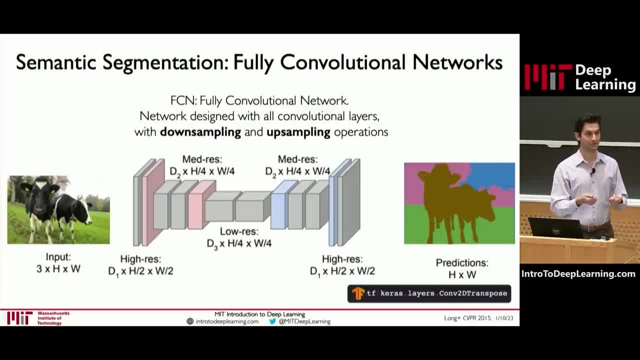 So instead of doing convolutions with pooling, you can now do convolutions with basically reverse pooling or expansions. Right, You can grow your feature sets at every labels And here's an example on the bottom of just a code piece that actually defines these layers: 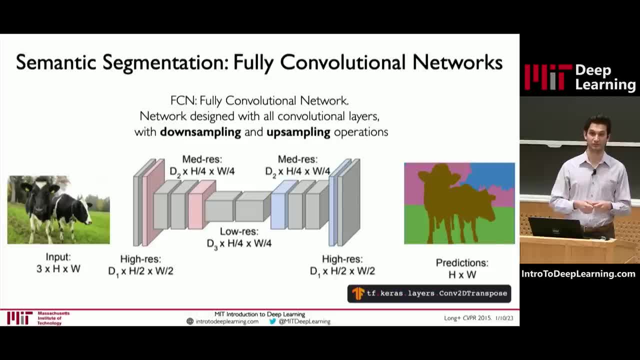 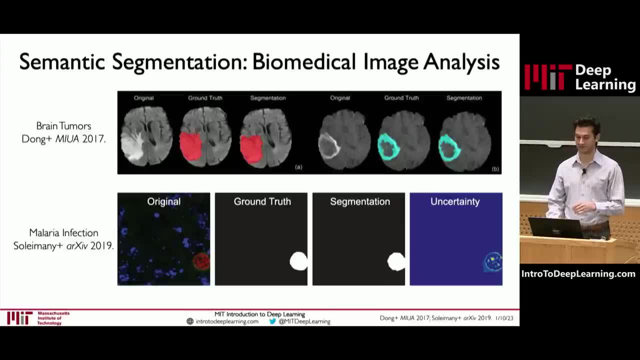 You can plug these layers, combine them with convolutional layers, And you can build these fully convolutional layers. You can build these fully convolutional networks that can accomplish this type of task. Now, of course, this can be applied in many other applications in health care as well, especially for segmenting out, let's say, cancerous regions, or even identifying parts of the blood which are infected with malaria, for example. 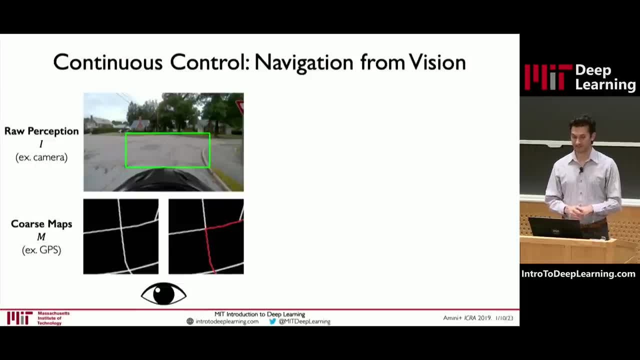 And one final example here of self-driving cars. Let's say that we want to build a neural network for autonomous navigation, specifically building a model, let's say, that can take as input an image As well as, let's say, some very coarse Maps of where it thinks it is. think of this as basically a screenshot of, you know, the Google Maps essentially to the neural network. 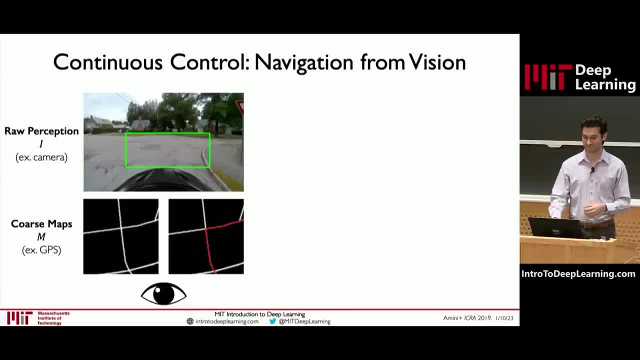 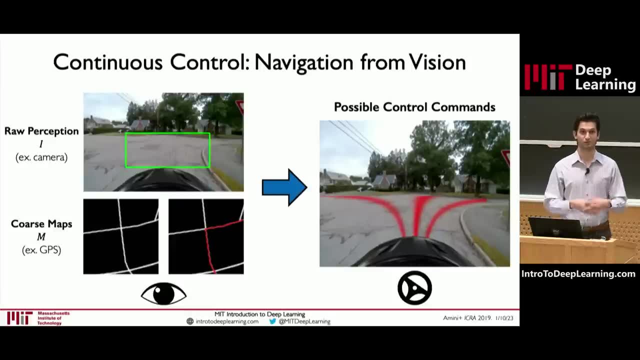 Right, It's the GPS location of the map And it wants to directly infer, not a classification or a semantic classification of the scene, but now directly infer the actuation: how to drive and steer this car into into the future. Right Now, this is a full probability distribution over the entire space of control cars. 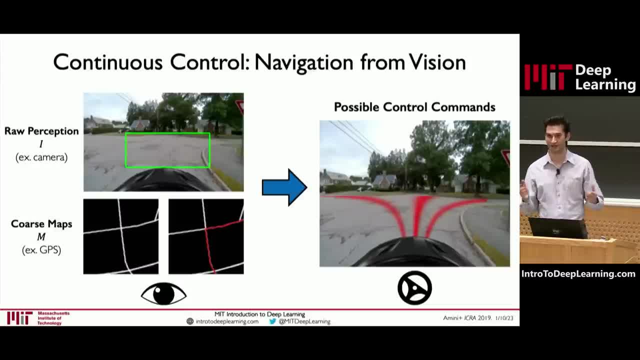 Right, It's a very large continuous probability space And the question is: how can we build a neural network to learn this function? And the key point that I'm stressing with all of these different types of architectures here is that all of these architectures use the exact same encoder. 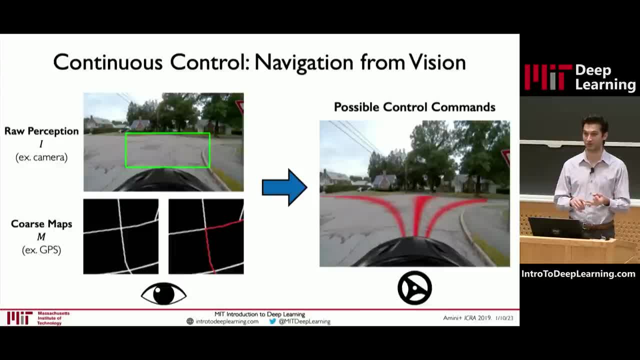 We haven't changed anything when going from classification to detection, to semantic segmentation and now to here. All of them are using the same underlying building blocks of convolutions, nonlinearities and pooling. The only difference is that After we perform those feature extractions, 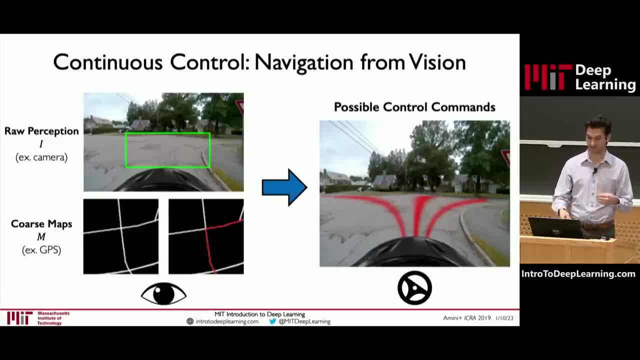 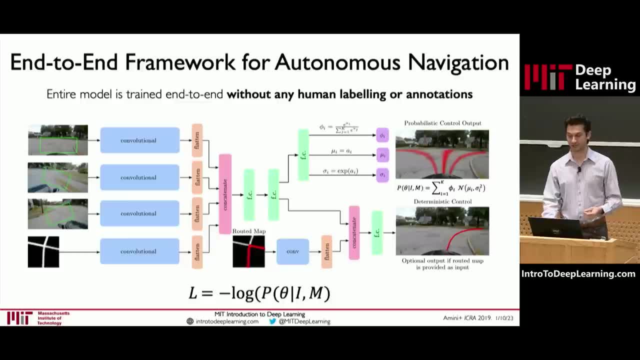 How do we take those features and learn our ultimate task? So, for example, in the case of probabilistic control commands, we would want to take those learned features and understand how to predict the parameters of a full continuous probability distribution, Like you can see on the right hand side, as well as the deterministic control of our desired destination. 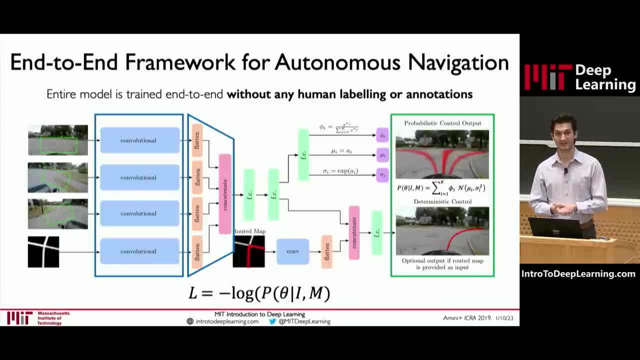 And again, like we talked about at the very beginning of this class, This model, Which goes directly from images all the way to steering wheel angles, essentially of the car, is a single model. It's learned entirely end to end. We never told the car, for example, what a lane marker is, or you know the rules of the road. 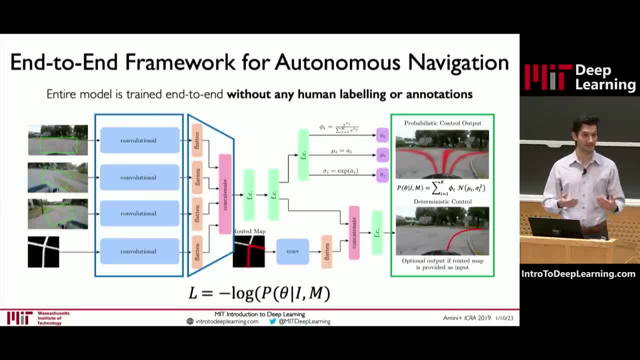 It was able to observe a lot of human driving data, extract these patterns, these features, from what makes a good human driver different from a bad human driver, And learn how to imitate those same types of actions that are occurring So that without any, you know, human intervention or human rules that we impose on these systems, they can simply watch all of this data and learn how to drive entirely from scratch. 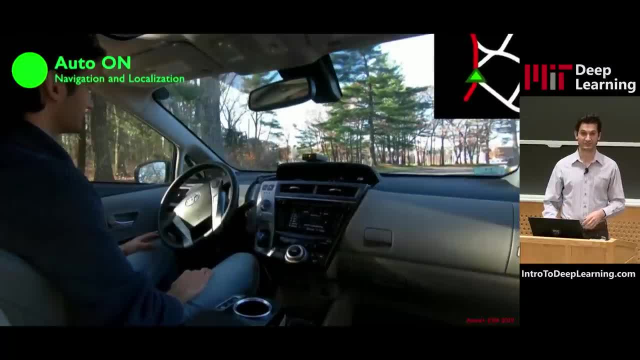 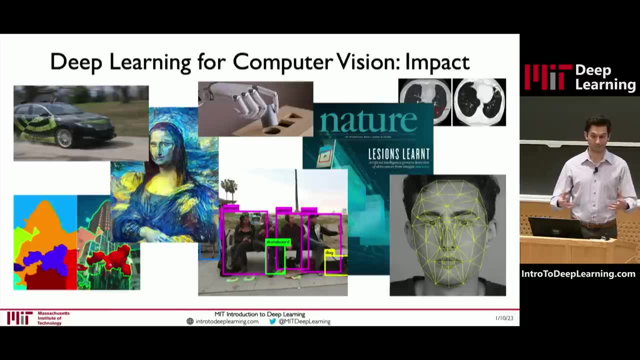 So a human, for example, can actually enter the car input, a desired destination, And this end to end, CNN will actually actuate the control commands to bring them to their destination. Now I'll conclude today's lecture With just saying that the applications 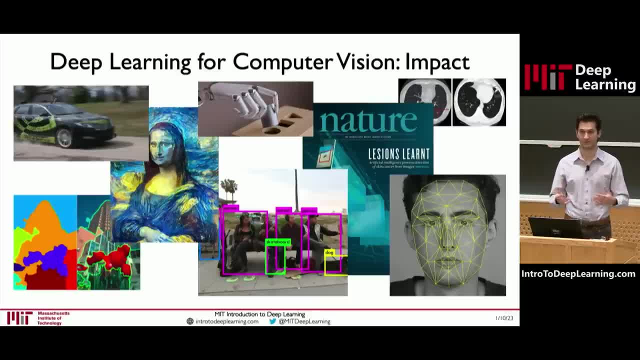 Of CNN's. we've touched on a few of them today, but the applications of CNN's are enormous, right far beyond these examples that I provided today. They all tie back to this core concept of feature extraction and detection And after you do that feature extraction, you can really crop off the rest of your network and apply it to many different heads, for many different tasks and applications that you might care about. 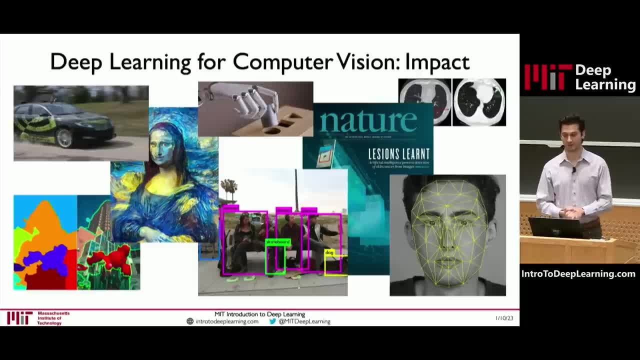 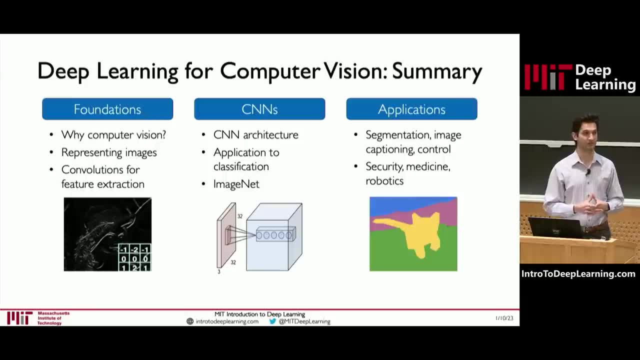 We've touched on a few today, but there are really so, so many in different domains, And with that I'll conclude, And very shortly we'll just be talking about generative modeling, which is a really central class, really central part of today's and this week's lectures series. 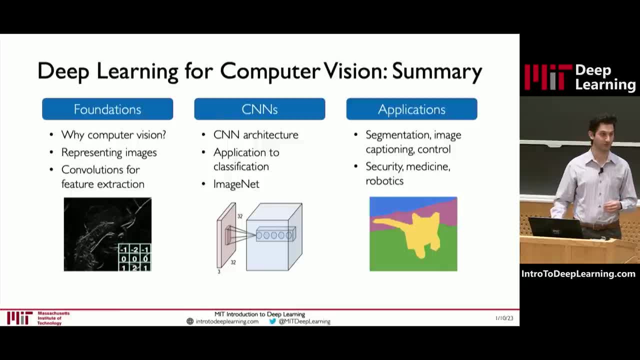 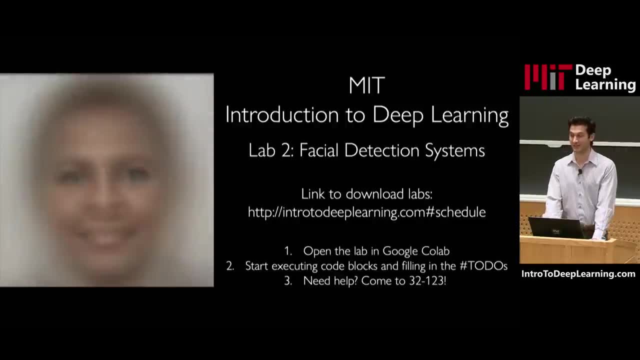 And after that, later on, we'll have the software lab, which I'm excited for all of you to start participating in. And, yeah, we can take a short five minute break and continue the lectures from there. Thank you, Thank you.